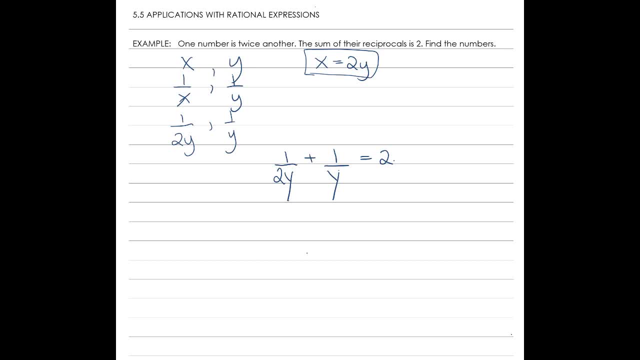 If you remember, we're going to multiply by the LCD. In this case, the LCD is 2y. Okay, so let's multiply. So this is 2y and then we'll subtract everything by 2y, Okay. 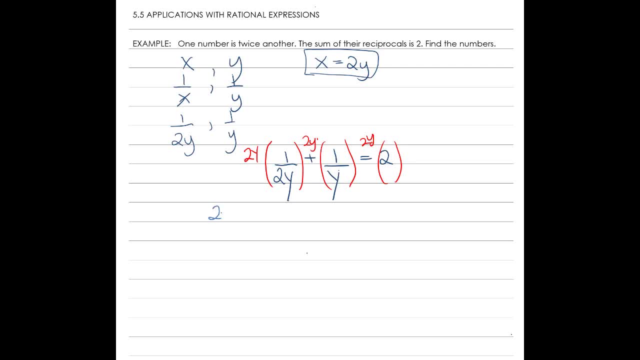 2y times 1 is 2y and that's 2y over 2y plus 2y times 1 is 2y over. y equals well, 2y times 2 is kind of 2y. 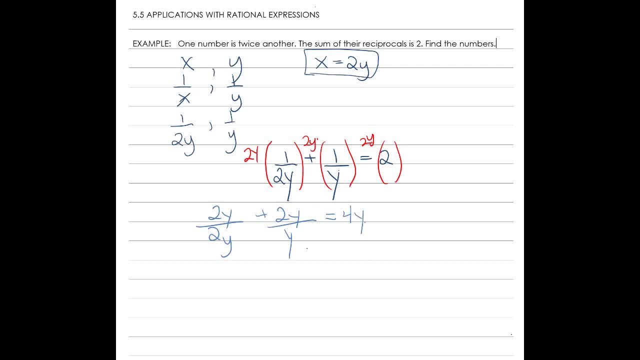 Okay, so that's 2y over 2y plus 2y times 1 is kind of 2y over y equals well, 2y times 2 is 2y is 4y. We can reduce some of this: 2y over 2y, well, 2y goes into 2y once, then 2y goes. 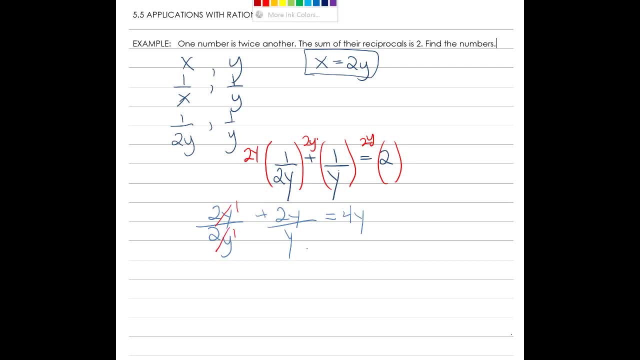 into 2y once, so that's just a 1. 1 plus well, y goes into y once, then y goes into y once, and 2 times 1 is 2.. That's 1 plus 2 equals 4y. so 3 equals 4y, and therefore. 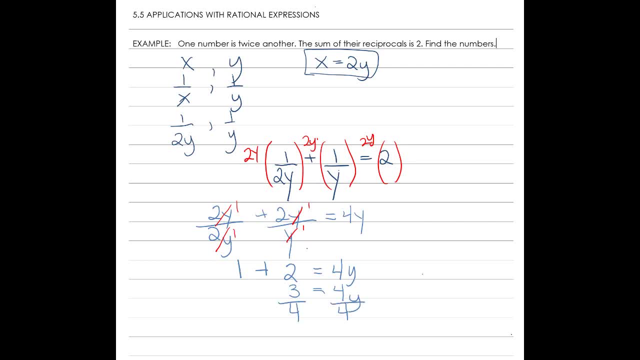 we're going to divide by 4,, divide by 4.. y equals 3 fourths. Now that we know what y is, we can solve For x. we can plug in what y is and say that x equals 2 times 3 fourths, And again. 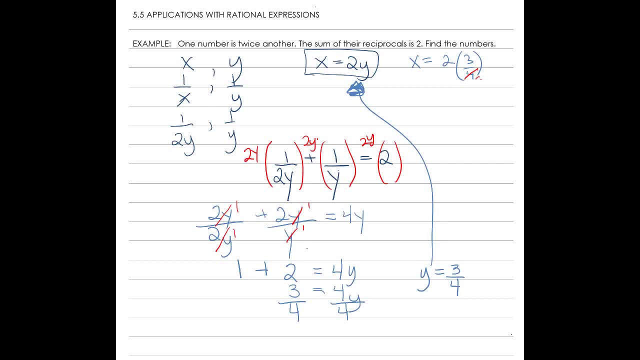 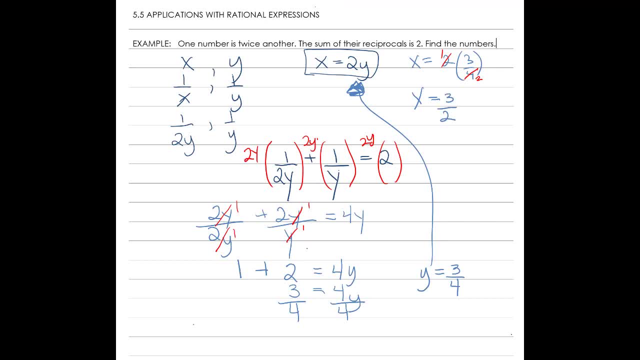 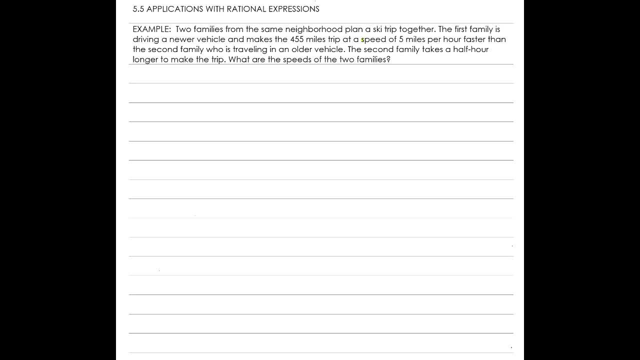 This time. let's say, two families are from the same neighborhood and they are taking a ski trip together. The first family is driving a newer car and makes the 455 mile trip at a speed of 5 miles per hour faster than the second family, who is driving an older car. 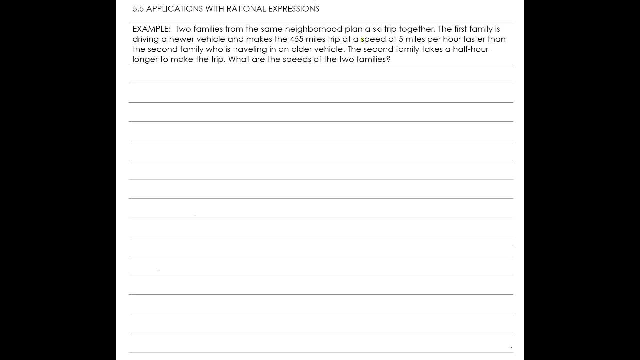 The second family takes a half an hour longer to make the trip. What are the speeds of the two families? One of the first things we need to figure out is what's the important information that we need to be able to solve this problem. There's a lot of information. 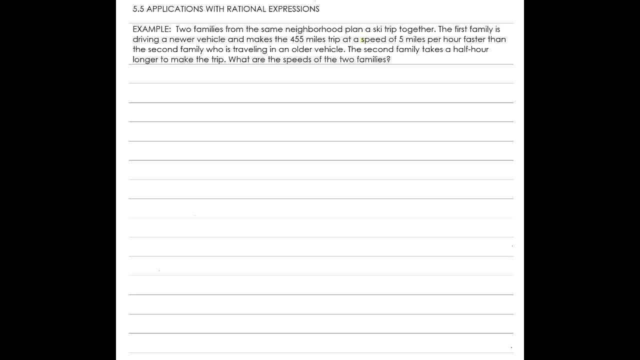 that's in this problem that we don't care about. We don't care that they're from the same neighborhood and we don't care that they're going to ski trip together. We don't even care if one vehicle is newer than the other. 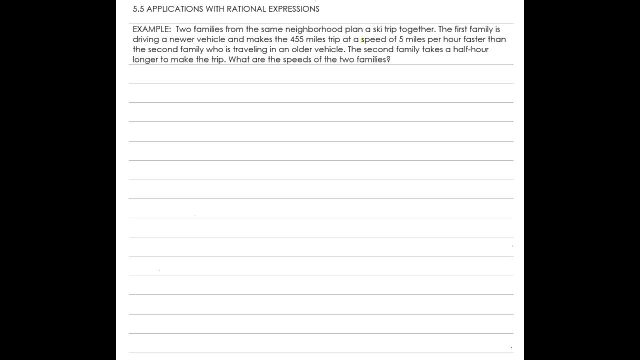 That has no bearing on solving what speeds they were traveling at. So here's what's important: The distance they drove- 455 miles- That's important. The speeds at what they traveled- well, the fact that one speed was 5 miles per hour than the other is important. 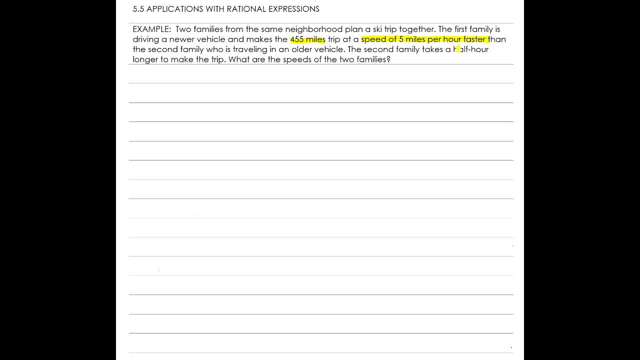 It's also important that one of the families took a half an hour longer to make the same trip. That's the important information here. The rest of it, at least to solve what we're looking for, is irrelevant. This is a distance equals. 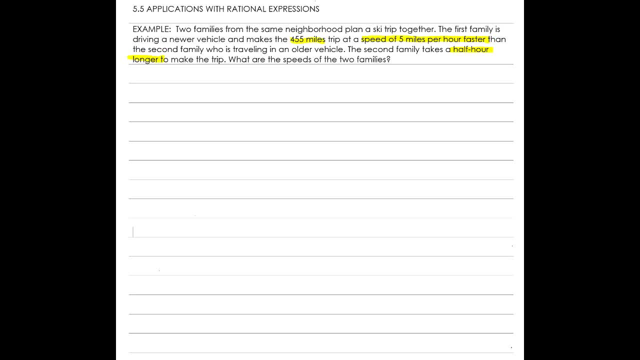 the rate of speed times a time problem. So distance equals rate of speed times time. That's what this problem really is. It comes down to distance equals rate times time. We are dealing with two groups of people: The first family and the second family. 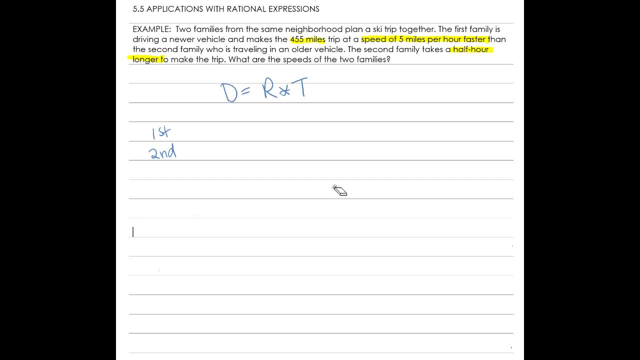 Okay, Here's what we know. I'm just going to make a little box here. Let's try that one more time. Okay, We know the distance will equal the rate of speed times the time. We also know their distances are 455. 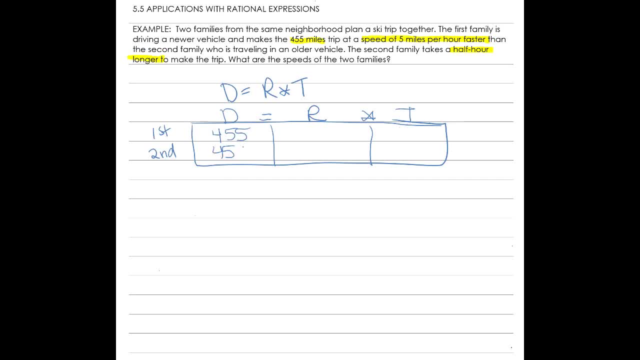 miles per hour. Sorry, 455 miles. Both of them travel 455 miles. We also know the first family drove 5 miles per hour faster than the second family. We don't know how fast the second family drove, So I'm just going to say they drove. 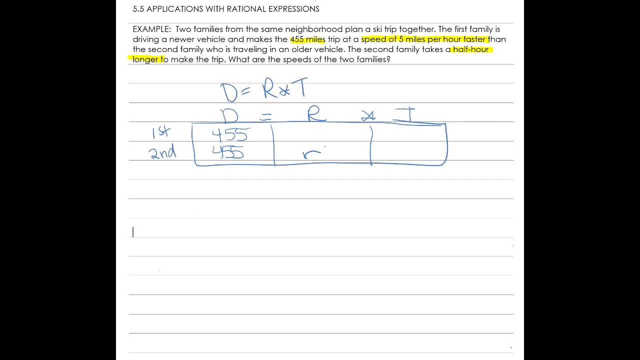 the rate of speed of r, And that means the second family drove 5 miles per hour faster. so that's r plus 5. Time- That's the only thing left. we have to fill in here The time We know that the 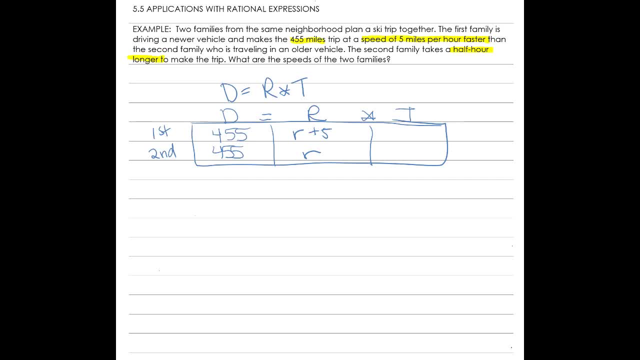 second family took a half an hour longer than the first family. We don't know how long the first family took, So I'm just going to call that t, And I know the second family took a half an hour longer than that. So we'll say that's t plus 1 half. 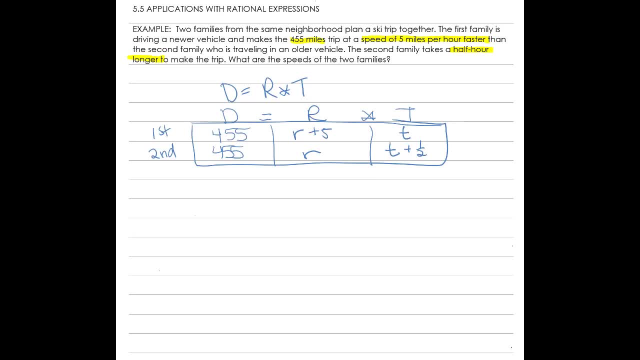 Okay, We have two equations and two unknowns. We can solve this. First equation: 455 equals r plus 5 times time. That is their equation. The second family's equation is: 455 equals their rate of speed times their time, which is t plus 1 half. 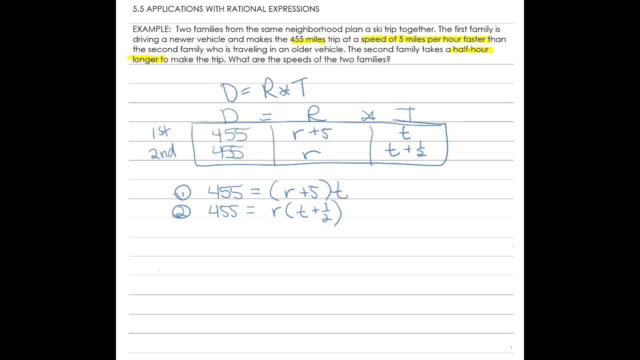 Okay, We're nearly there. Well, at least in terms of setting it up, we're nearly there. We have two equations. We just need to figure out how are we going to solve these. The first equation we could solve for t: 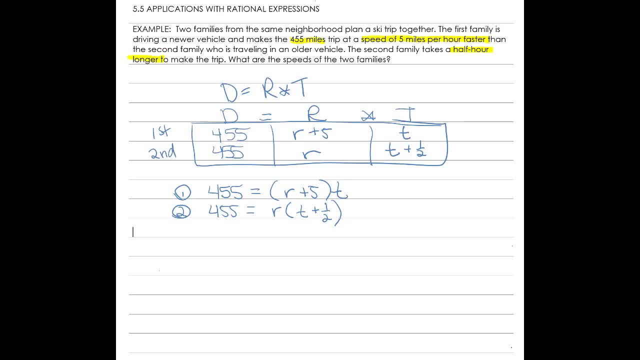 And then plug it into the second equation. So that's one option: Solve the first equation for t And then plug that into the second equation, And then we could solve for r. The other option is: solve the second equation for r And then plug that into the first equation. 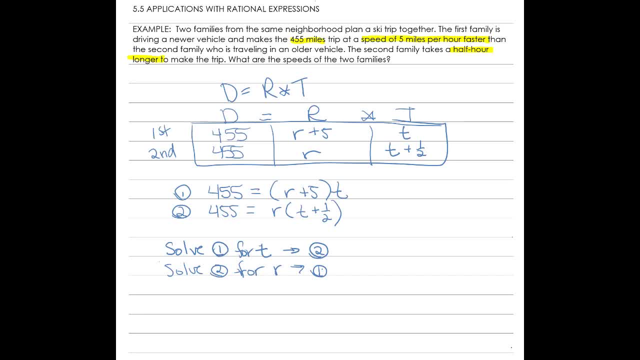 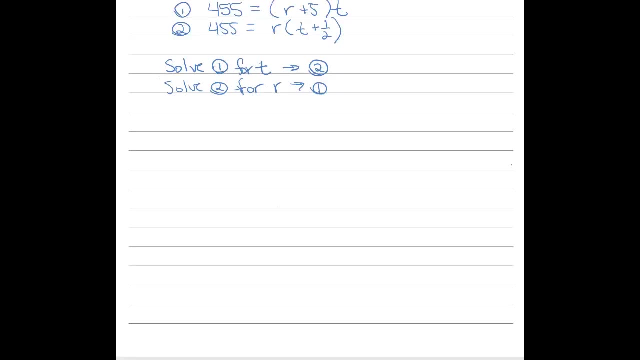 And then we would solve for t and back substitute to get the actual value of r. Now I'm going to go with the first option. So hang on tight, Let's get this going Alright. so I've given myself a little bit more space here. 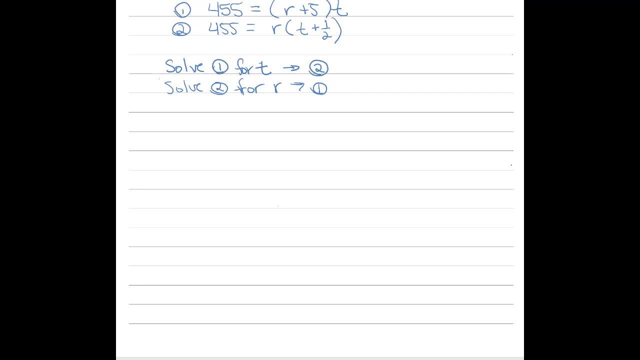 And I think I am going to solve the first equation for t And then, whatever I get for t, I'm going to plug it into the second equation. So number one, Let's solve for t. Alright, 455 equals r plus 5 times t. 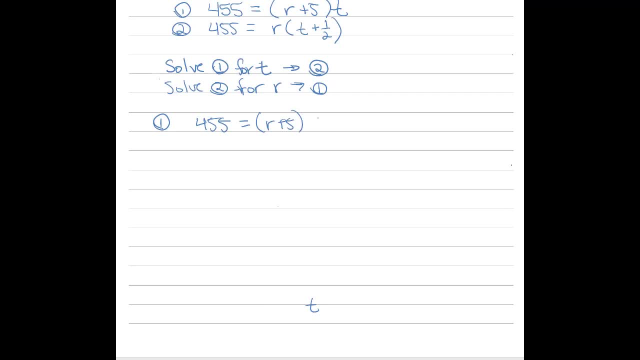 The good part about this is that it's relatively simple to solve for t, Because all I need to do is divide the right hand side by r plus 5.. What I do to the right hand side, I need to divide by the left hand side as well. 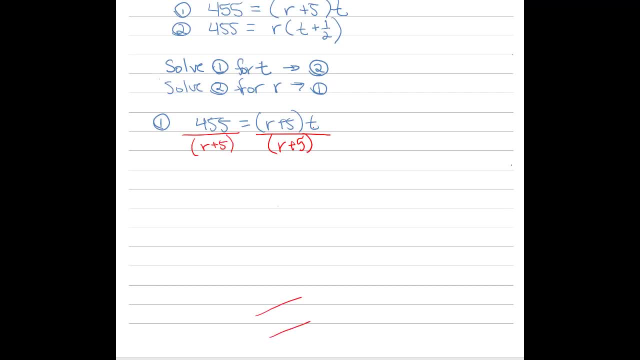 r plus 5.. Alright, so now we know what t equals. t equals 455 over r plus 5.. So we know t. Now that we know t, let's go ahead and plug this value into the second equation. So here's our new number 2.. 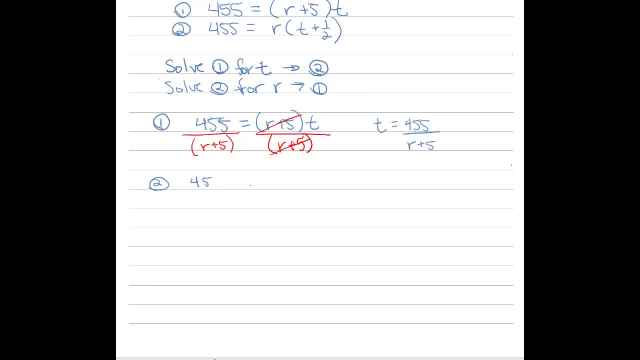 455 equals r times our new t value, Which is 455 all over plus 5 plus 1 half. Okay, Let's take a look at what we have now. It is quite complex, but it is solvable. What I would like to do: 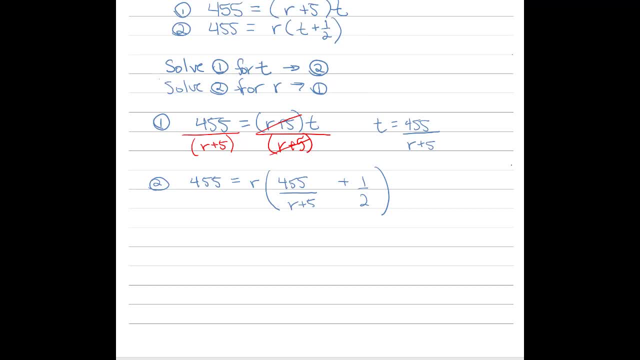 is using the parentheses. I want it under one fraction. I think this will help us a little bit in terms of solving this. So I'm just going to do common denominator and add those two fractions together. My common denominator is going to be 2 times. 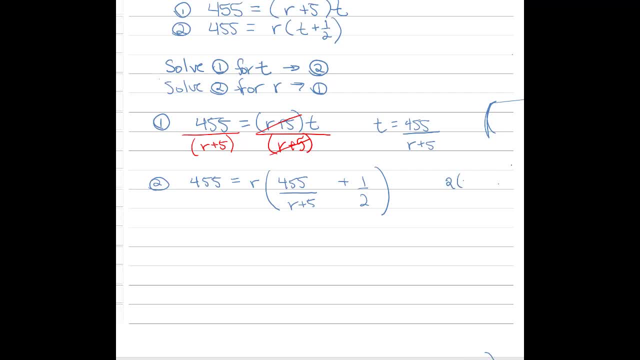 r plus 5.. 2 times r plus 5.. Okay, So I need a 2 times r plus 5 here And a 2 times r plus 5 on our second term, And then that will give us common denominator and see: 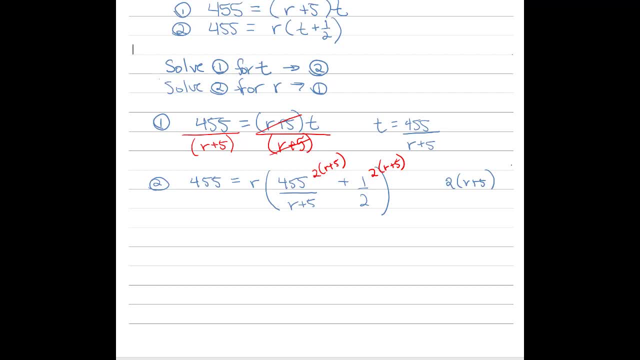 actually I don't need to do that part. I actually just need to multiply this first fraction because it already has the r plus 5.. I just need to multiply that one by 2.. 2 over 2. Because 2 over 2 is just a nice. 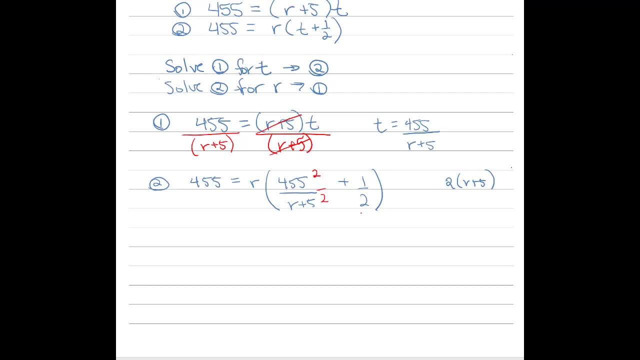 little 1.. So 2 over 2.. And for the second fraction it needs the r plus 5. And we'll do r plus 5 over r plus 5.. And that is a nice 1.. Okay, So this new. 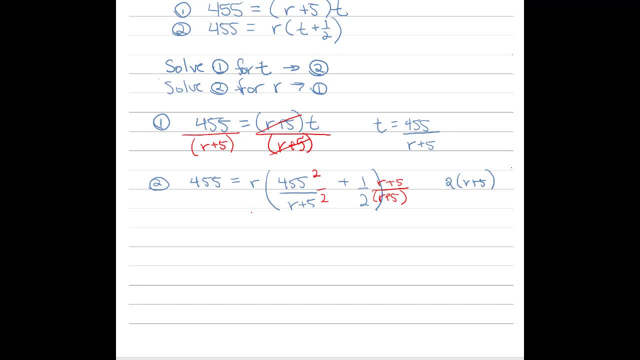 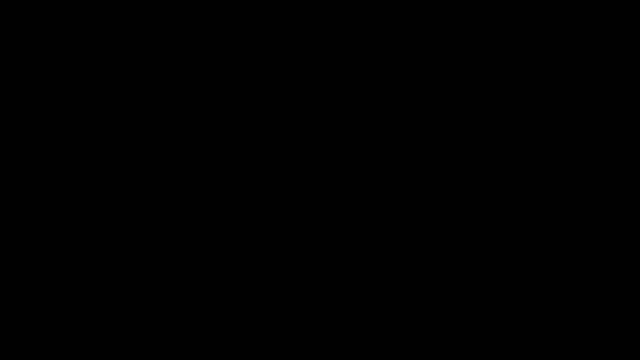 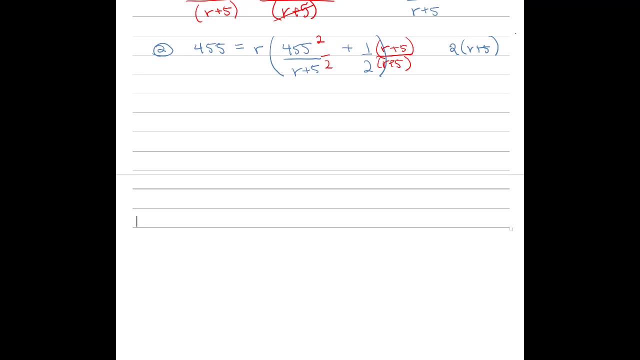 parentheses will be Okay. So now that we have common denominator, it will be: 455 equals r times all under the same common denominator of 2 times r plus s, r plus 5, pardon me, And we have 2 times 455, which is 910. 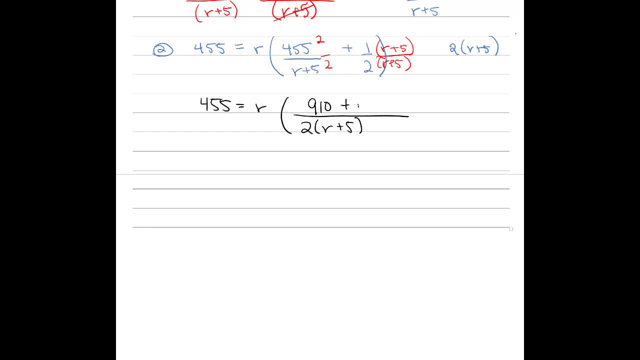 plus well, 1 times r plus 5 is r plus 5.. Okay, We could add the 910 and the 5. together, It's going to be 455 equals r times 915 plus r all over. well, I'm going to go ahead and do that math. 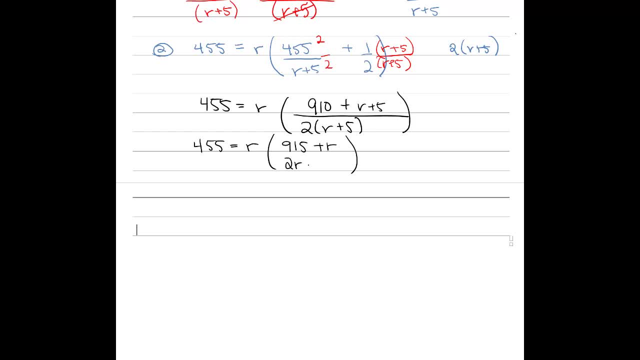 of 2 times r is 2r, and 2 times 5 is 10.. Okay, So now here's what I'm going to do. I'm going to get rid of that fraction by multiplying both sides by 2r plus 10. 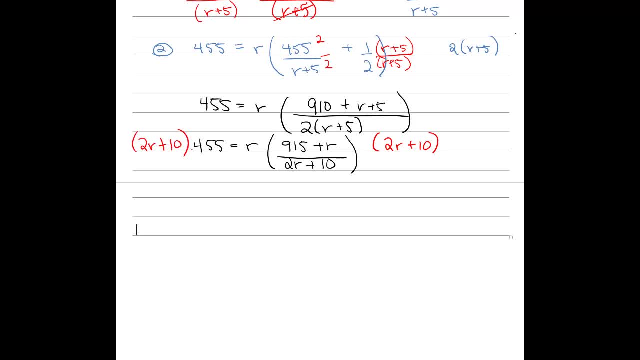 and 2r plus 10.. Once I do that, the fraction on the right will go away and we are left with 455 times 2r plus 10 equals r. well, that's not lining up very nicely. Let's move it down just a wee bit. 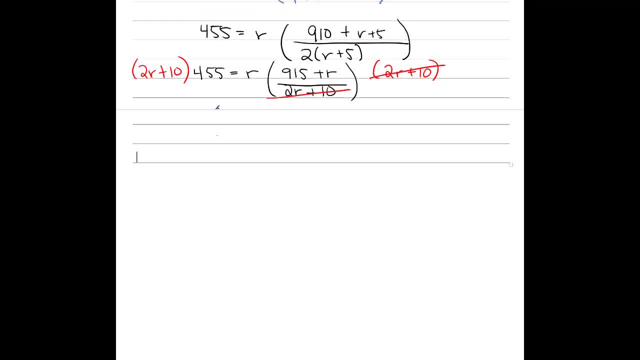 Okay, Let's see if that's the issue. Okay, So we have 455 times 2r plus 10 equals r times 915 plus r. Okay, We're getting there Now. I've got r's all over the place. I've got numbers. 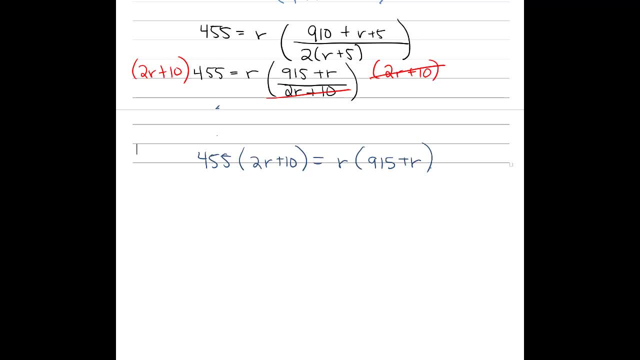 all over the place. I'm going to go ahead and distribute. I'm going to get everything on one side. I'm going to factor and then see what I get. Okay, Distribute 455 times 2r is 910r. 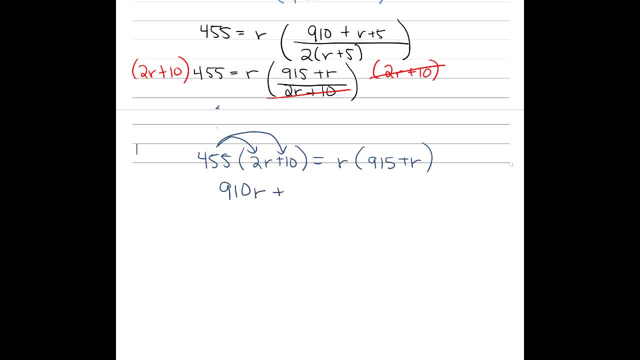 times 2r plus 455 times 10 is 4550, r times 915 is 915r, and r times r is r squared. Okay, r squared is positive. So I'm actually going to move everything to the right to keep that r squared positive. 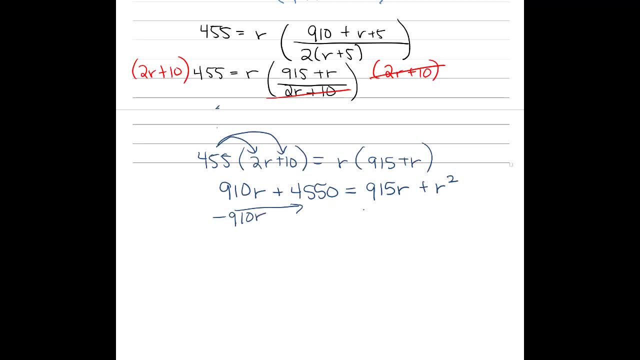 So, subtract 910r, subtract 910r, I'm left with 4550 equals 5r plus r squared. I'm going to subtract the 4550 from both sides, Oops, And that's going to give me 0 equals negative 4550. 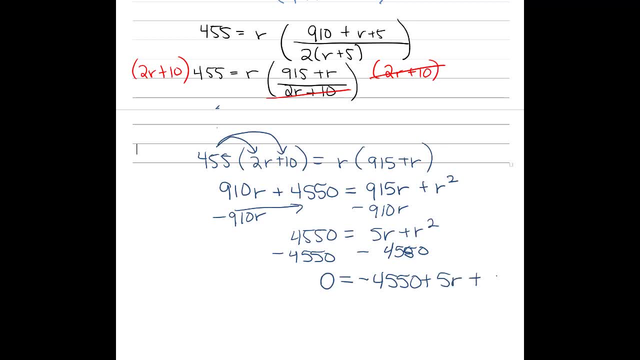 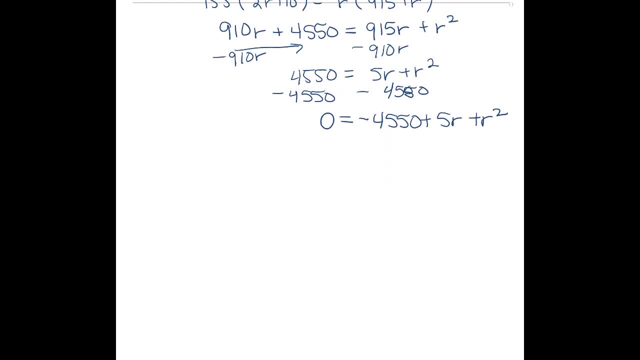 plus 5r plus r squared. Okay, It's a little awkward, so I'm going to rearrange this. Put everything on the left, Just switch the side of the zero and everything else. So r squared plus 5r minus 4550. 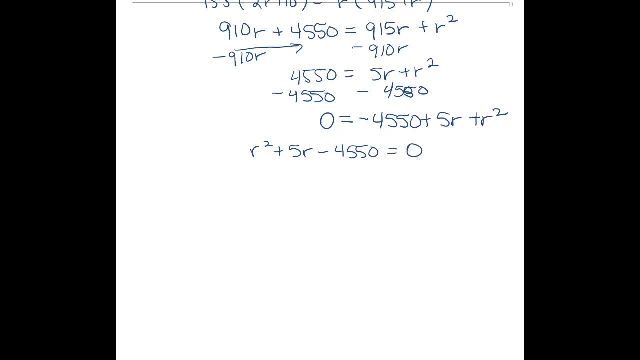 equals 0.. Now, with a little finagling, you will be able to factor the left hand side, r times r will give us r squared. We need two numbers fairly close together because when you one's negative and one's positive, that once you take the difference of these two numbers 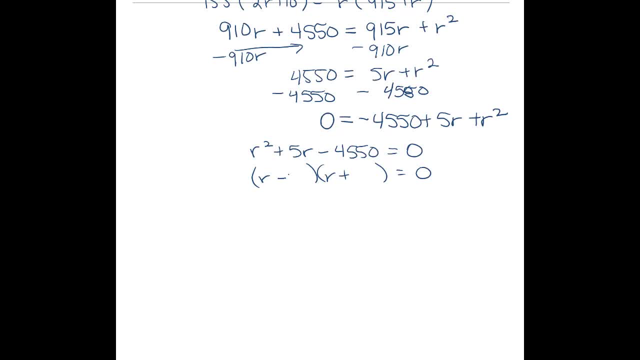 there's only 5 separating them And it turns out it's going to be 70 and 65.. r minus 70 equals 0. And r plus 65 equals 0. And we're going to solve for these values of r. 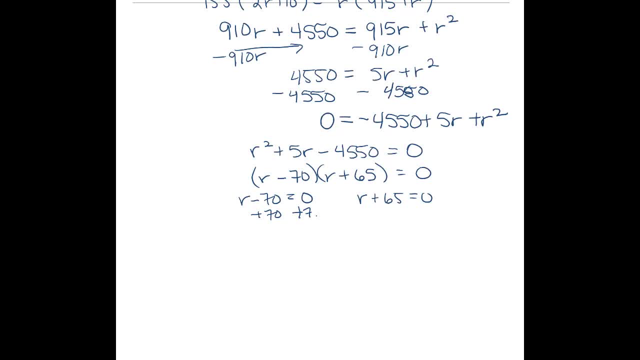 Add 70 to both sides, r equals 70. Remember, r is a rate of speed, so that's miles per hour. So subtract 65, subtract 65. r equals a negative 65 miles per hour. Can we have a negative speed? 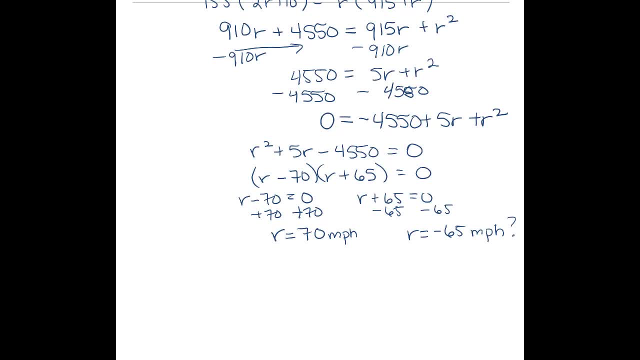 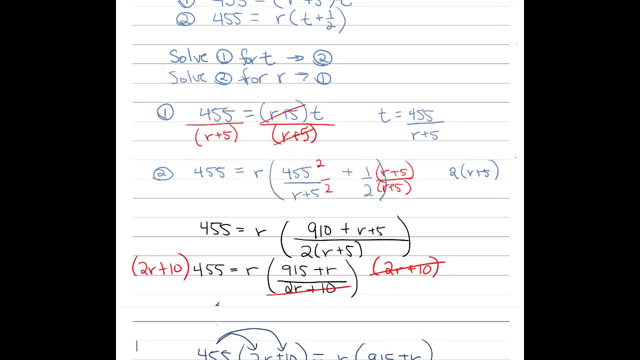 Well, mathematically it works out, but in reality, for the context of this problem, a negative speed doesn't make sense. So we found our speed of 70 miles per hour And I'm going to scroll up. our r was the rate of speed of the. 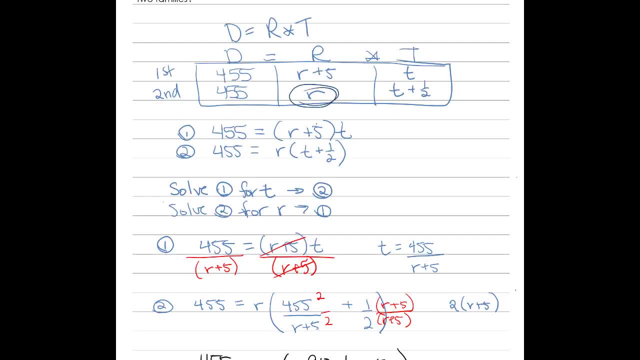 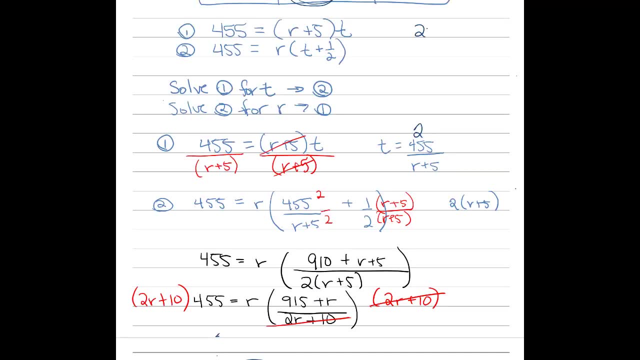 second family. r is the rate of speed of the second family. So the second- come on pin second family drove 70 miles per hour. The first family drove well, r plus 5.. So that's 70 plus 5. So their speed was 75. 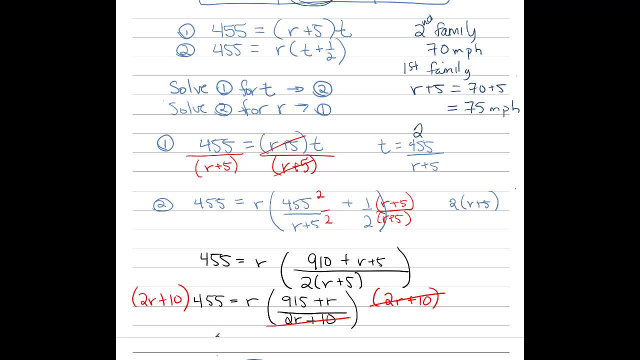 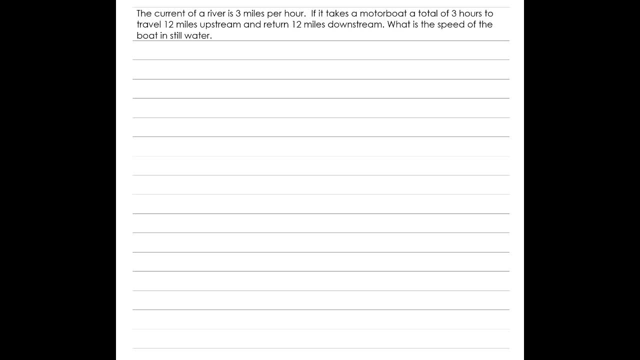 miles per hour. There are the two speeds. Let's take a look at another problem. The current of a river is 3 miles per hour. It takes a motorboat a total of 3 hours to travel 12 miles upstream and return the 12 miles downstream. 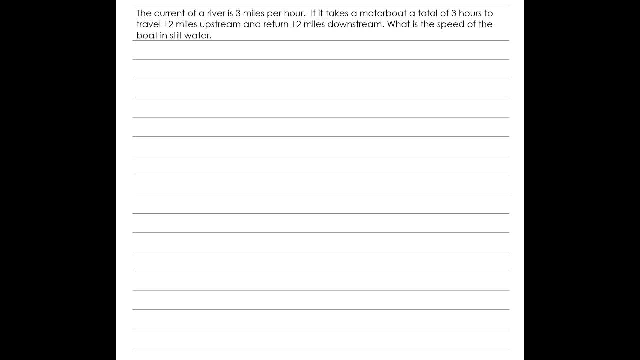 What is the speed of the boat in still water? Now, you may not ever go on a boat, or you may not ever think of this problem and have to solve it in the future, but there are a lot of things in the world that takes into effect. 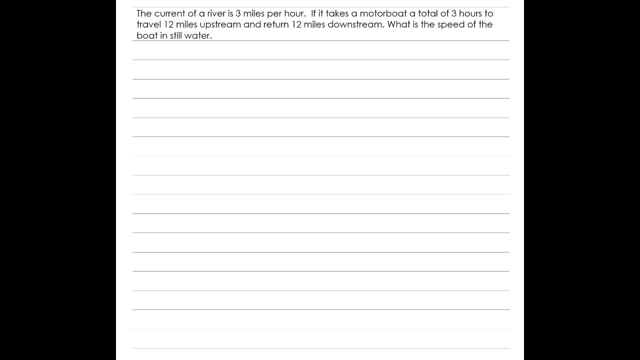 something going against you. So let's say it's a really super windy day and you're running into the wind. Well, that's going to be pushing against you and you're going to have to exert a lot more energy to race against the wind versus if the wind. 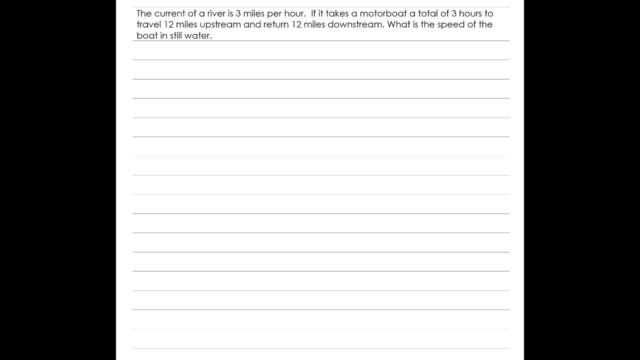 was at your back, then you can run a lot faster because the wind is actually helping you. Likewise, if you're in a plane and you have a headwind, which is going against you, versus a tailwind, it's going with you. Same thing in a. 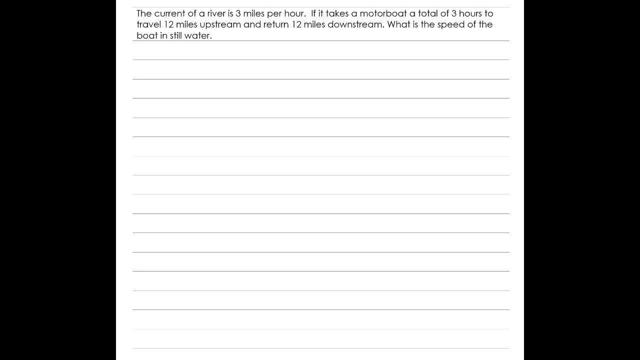 car. Wind plays a very important matter in dealing with fuel economy. The other thing is, when you're in a boat, well, what's playing against you? there is not necessarily wind, so much as the current of the river or current of the lake or current of the ocean. 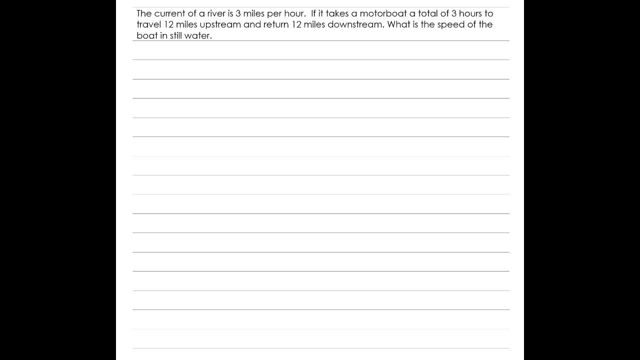 And it takes a lot more energy to go against the current than it does to go with the current. Alright, so here's the important information. number one: the current is three miles per hour. I'm just going to write that, as C equals three miles per hour. 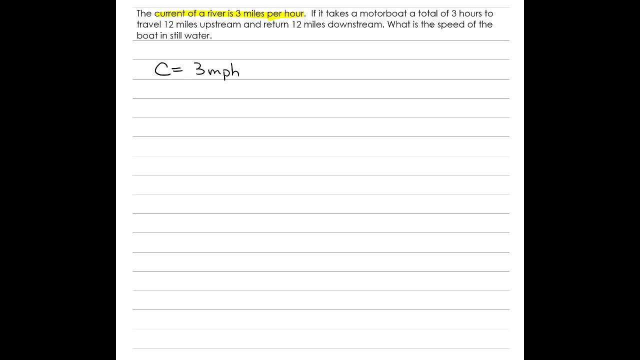 We also know the distance the motorboat goes is twelve miles. Not only does it go upstream twelve miles, it also goes downstream twelve miles. And then we know that it takes that whole entire trip, the whole entire time, to travel three miles, both upstream. 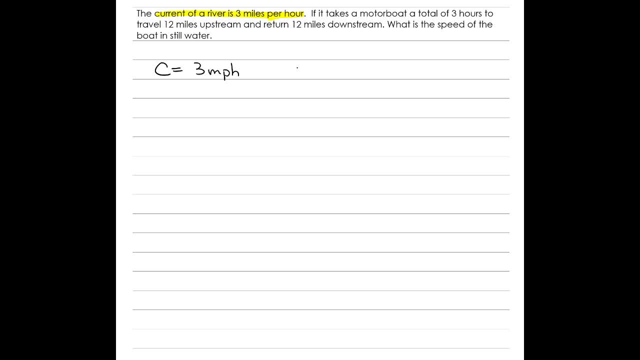 and downstream. So let's put all this together. This is a distance, time rate, times time problem. still, We have some speed upstream and then we have downstream. we have some information downstream. Okay, The distance in both cases is twelve. We go upstream twelve. 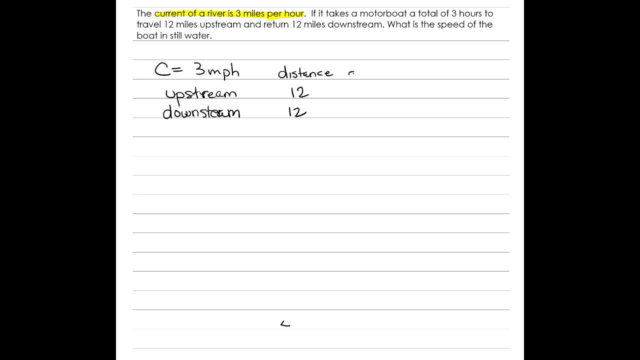 and we come back twelve miles downstream. Now the distance will equal the rate, of the speed times the time it takes. Now here's the thing: When you are going upstream against the current, The current is not helping you. In fact, it's hurting you. 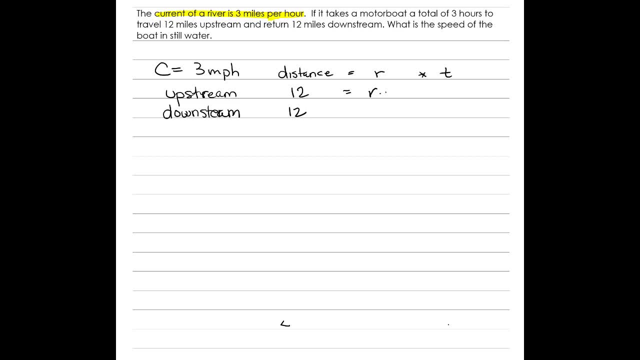 So your rate of speed is going to be your rate of speed minus the current. It's going against you. Likewise, or anti-likewise, if you are going downstream, the current is with you. It is helping you, So it's going to be your rate of speed. 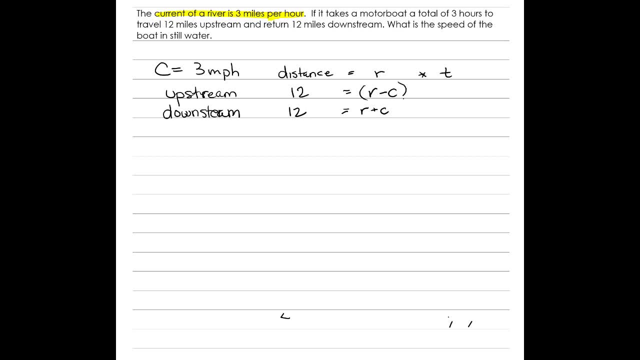 plus the current is going to be your speed. Alright, Now the time up and the time down are going to be two different times. For now I'm going to label it time up and time down. Okay, So we're getting there Now. 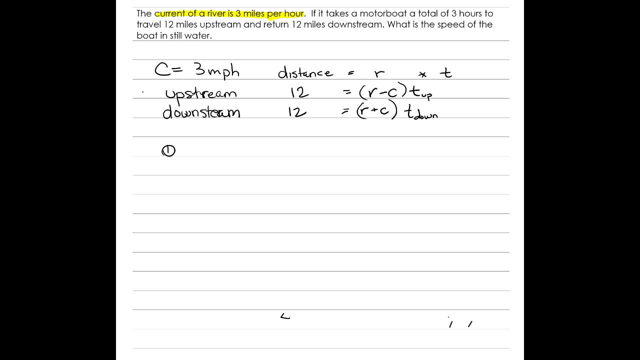 let's also take into consideration. so that's going to be one, two and this is going to be our third one. We also know our time up plus our time downstream- let's do that right time down. well, that whole trip takes three hours. We also know 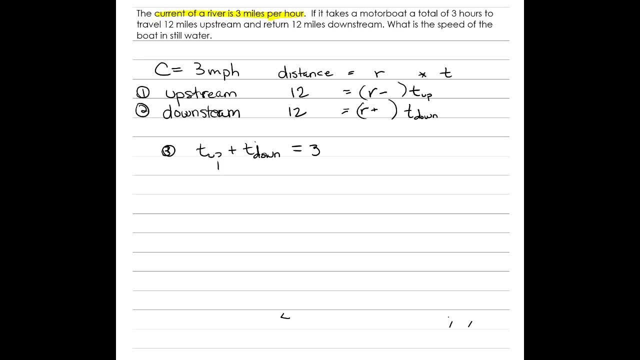 our current is three, So I'm going to replace the c with our three miles per hour. that we know our current is Okay. If I solve, let's solve the first equation for time up and then we'll solve the second equation for time down. 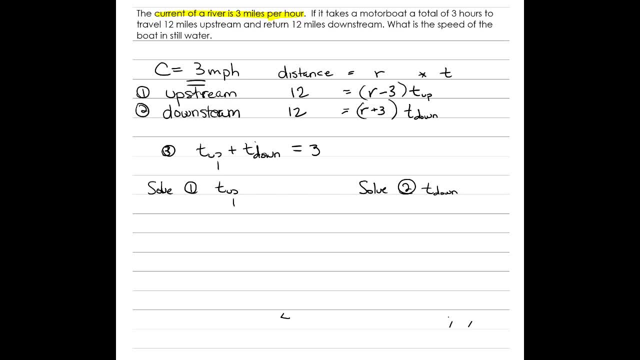 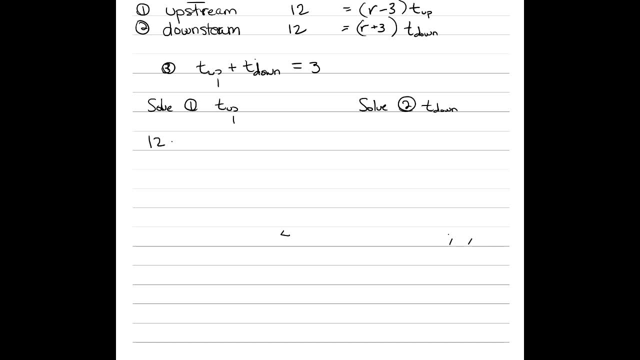 And then we can plug them into our third equation and get something that we'll be able to solve. Okay, Twelve equals r minus three versus the time up. Let's divide each side by r minus three, divide by r minus three, so time up will equal. 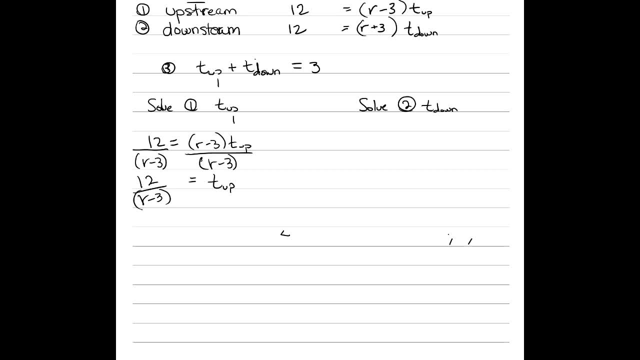 twelve over r minus three. Okay, We've got that so far. Similarly we have for the time down. we have twelve equals r plus three times the time down. we're going to solve this for time down by dividing by r plus three on both sides. 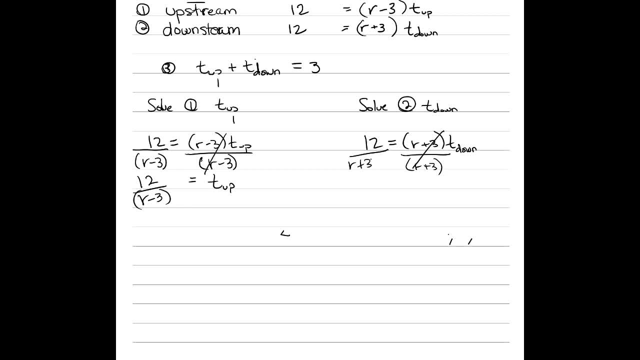 r plus three on both sides and we get twelve over r plus three will equal our time down. Okay, We have everything we need. We're going to use the third equation and plug in our time up and plug in our time down and solve for the equation. 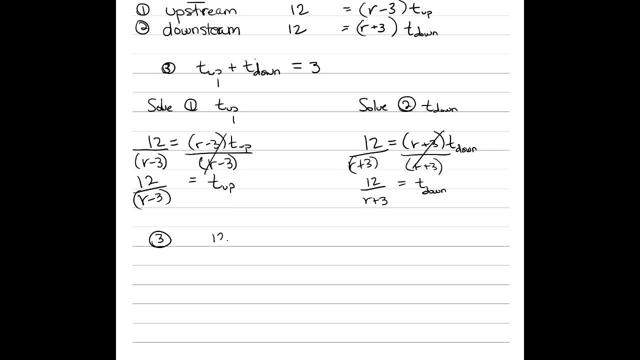 So in our third equation we have time up twelve over r minus three, plus our time down, twelve over r plus three. that equals three. I just want to fix that parenthesis a little bit here so it looks more like a parenthesis to you. Okay, We only have one unknown. 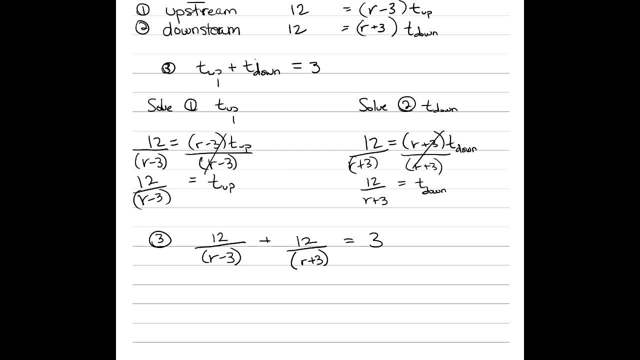 We're going to solve for the rate of speed. Alright, To get rid of those fractions, we're going to multiply both sides by the LCD. In other words, I'm actually going to multiply every term by the LCD, And the LCD is r minus three. 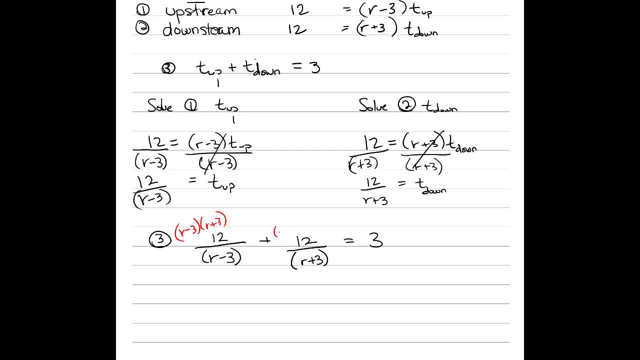 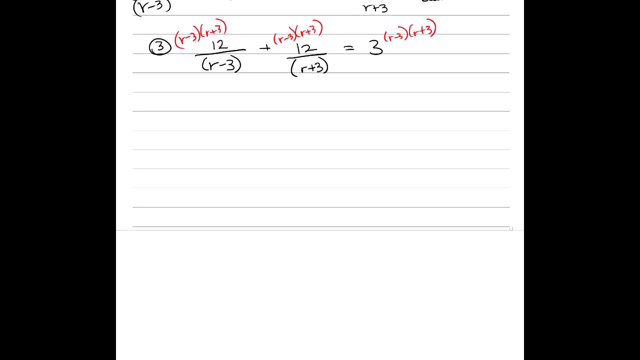 r plus three, And I'm going to multiply that to each term. And finally, r minus three, r plus three. Okay, Let's move that down so we have a little bit of space here. I'll use a different color just to reduce things. 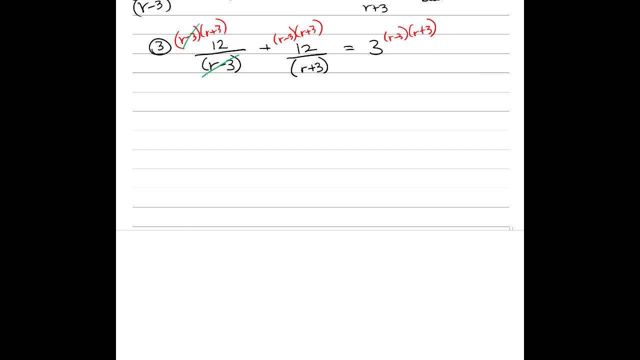 Alright. R minus three cancels out r minus three. R plus three cancels out r plus three. And here's what we've got left. Twelve times r plus three plus twelve times r minus three equals three times r minus three. r plus three. 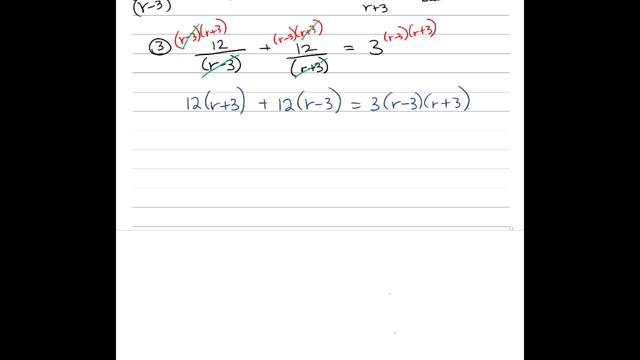 Okay, Let's distribute, Add like terms, Simplify as much as possible. So twelve times r is twelve r plus three times twelve is thirty-six Plus twelve times r is twelve r. Twelve times negative. three is negative thirty-six. And I'm going to 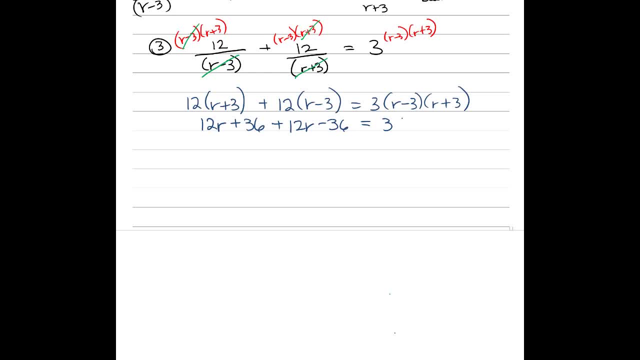 do the two parentheses first. That's going to be r squared minus nine. I'm going to add like terms: The thirty-sixes will cancel, and I have twenty-four. r equals three r squared minus twenty-seven. Alright, We are almost there. 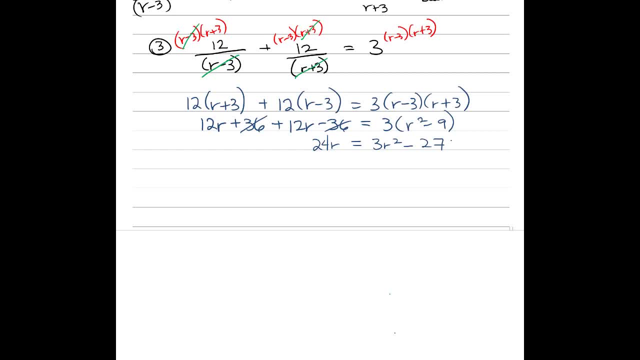 All we need to do is set this equal to zero factor, and then we will solve. Okay, So I'm going to move everything to the right. So I'm going to subtract twenty-four r. subtract twenty-four r- Zero equals. Come on Pin. 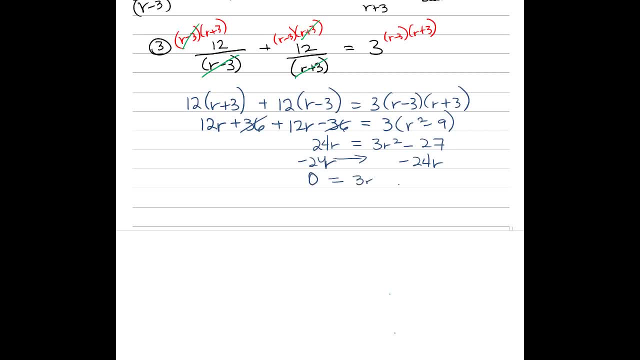 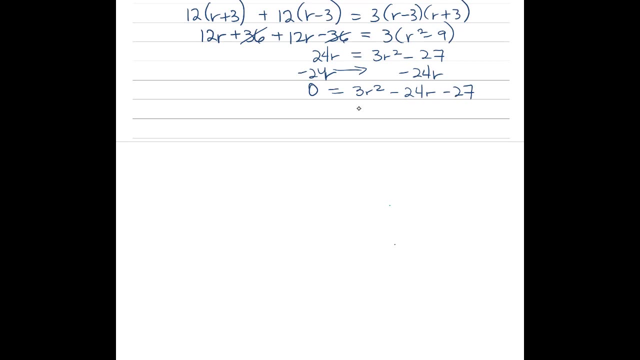 Zero equals three r squared minus twenty-four r minus twenty-seven. Now let's factor. First thing I can do is I can factor the three, the GCF. I'm not sure why it's not writing there, so let me try over here. 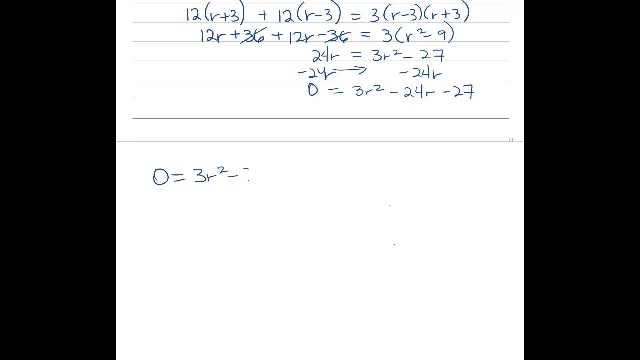 Zero equals three: r squared minus twenty-four, r minus twenty-seven. Let's factor out the three, leaving us with r squared minus eight, r minus nine, And that all equals zero. I'm going to go ahead and divide both sides by three. Divide. 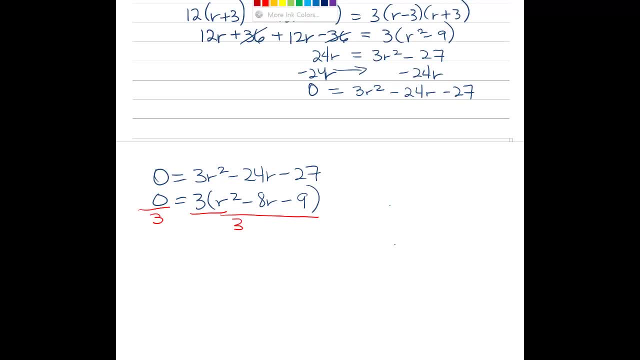 both by three, That will give us zero equals, not the color I want. Zero equals r squared minus eight, r minus nine. Let's factor: Zero equals r- r, Two numbers that multiply to negative nine. but add to negative eight, That will be a positive one. 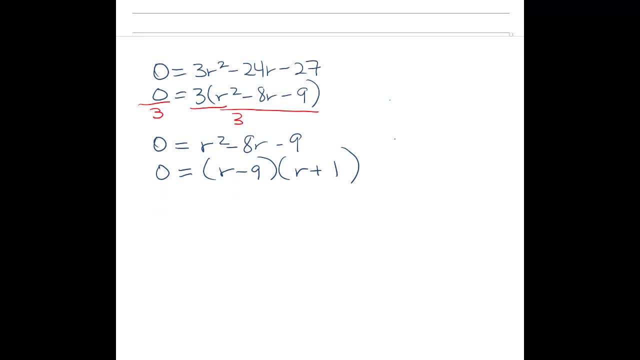 and a negative nine. Let's use the zero factor property: r minus nine equals zero And r plus one equals zero. For the first equation, let's add nine to both sides: r equals nine. Let's subtract one from both sides. 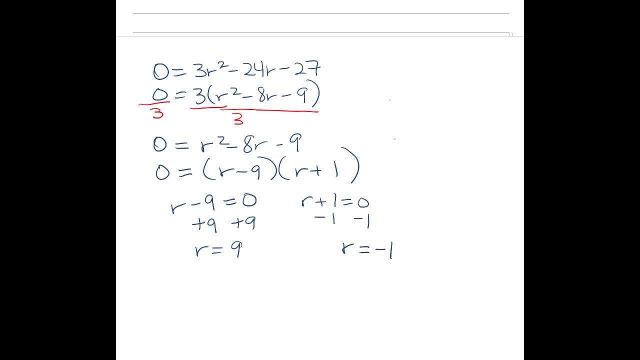 r equals negative one. We'll find that this is a rate of speed. Miles per hour. Miles per hour. A boat can go nine miles per hour. That is a good answer for this context. A boat cannot go a negative one mile per hour. 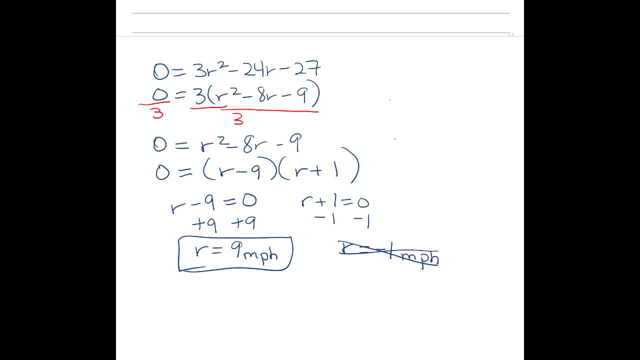 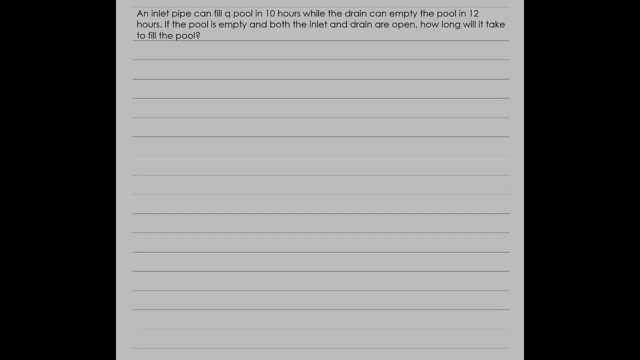 Although mathematically correct, it is not valid for this particular context. All right, let's try another problem, and this is an inlet pipe drain problem, and it's kind of a cool way of thinking about it. If you have, you can even think of this as a faucet on versus water draining out. 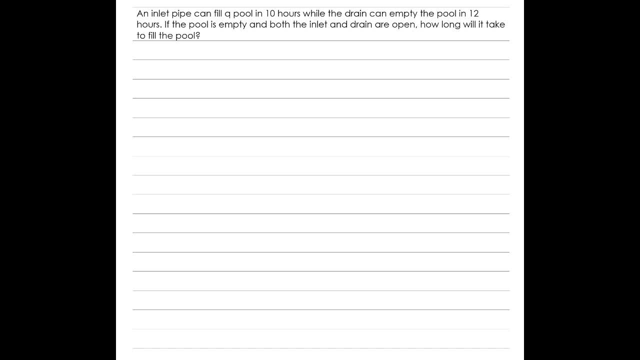 So I know this is a pool, but I can't really draw a pool with a drain and an inlet pipe, So I'm going to go ahead and just draw a tub. So let's say we have a pool like a kiddie pool, and it has- oh, I don't know. we'll say 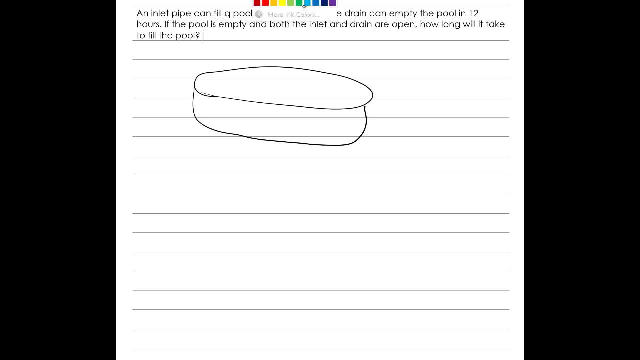 that it has a pipe coming in, a hose. we'll say like a, you know, like a water hose coming in and it's filling up with water. Okay, that fills it up with water. And then, likewise, unfortunately, somebody forgot to do the plug and the plug is down. 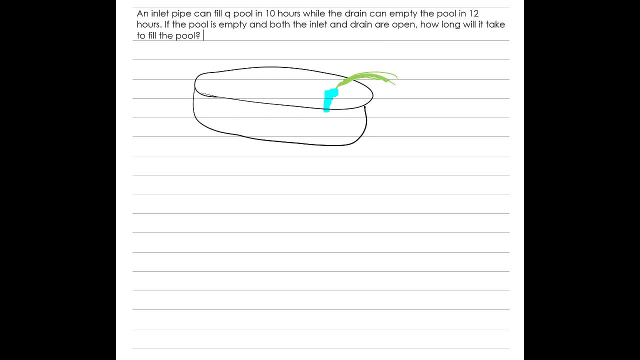 here and the water is seeping out as you fill it up. Okay, so as you're putting water in, it's also flowing out at the same time. Now you, If, If the drain was plugged, you could fill the pipe. you could fill this pool up in 10 hours. 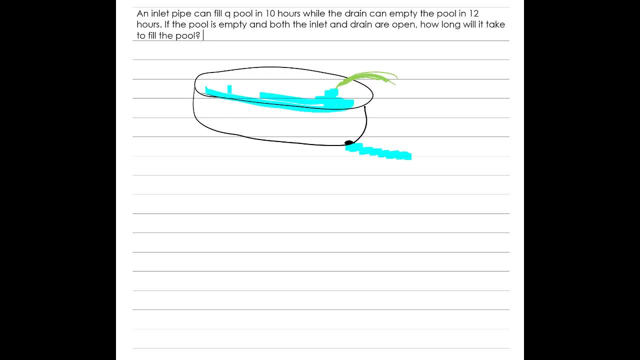 So here's the water on the inside of the pool. You could fill up this pool in 10 hours, And if the pool was completely filled and you let the drain out, it would drain in 12 hours. Okay, so here's the thing. 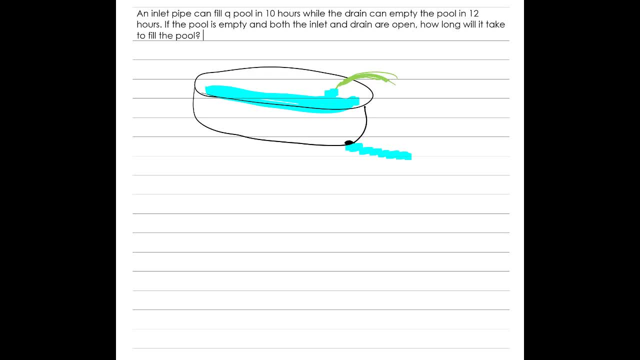 Let's say you leave them both open. So an inlet pipe, In other words the hose can fill a pool in 10 hours while it takes, the drain can empty the pool in 12 hours. If the pool is empty and both the inlet and the drain are open, how long will it take? 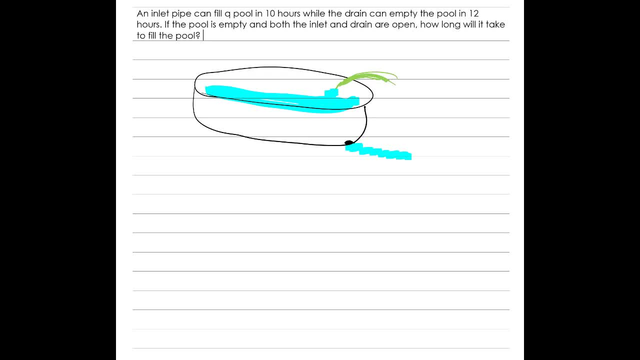 to fill the pool. First thing is: can we fill the pool? Yes, because it takes a shorter time to fill the pool than to empty the pool. So therefore it will eventually fill up. Not too sure how long it will take, But it will. 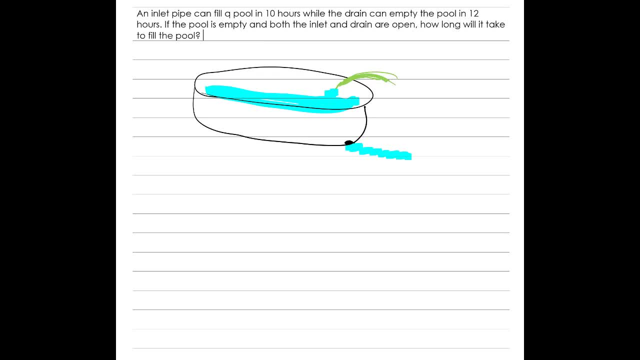 It will only eventually fill up. Now let's let x represent the time it takes to fill the pool. Fill the pool. What's the time it takes to fill the pool It takes? What's the time it takes to fill the pool? 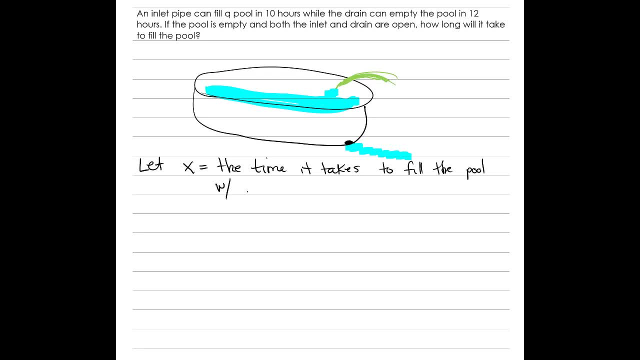 What's the time it takes? We're going to move forward with both the faucet on- I'm just going to call it the inlet open and drain open, Okay, so that's how long it's going to take to actually do it. We don't know. 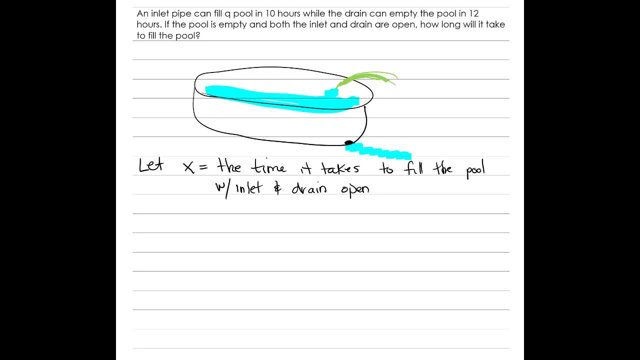 But it will happen. So we want to know How much. How much. I'm sorry of the pool. if we only had the faucet running but the plug in the drain so nothing was coming out, how much of the pool would fill in one hour? well it. 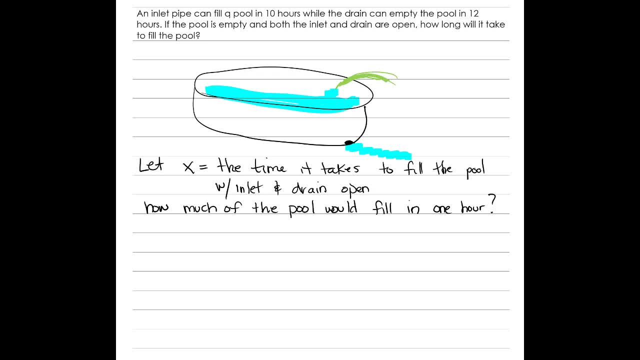 takes ten hours to fill it. so, therefore, in one hour it would be filled one tenth of the way, because it takes ten hours to fill it, and in the second hour it would be two tenths filled. third hour would be three tenths filled. fourth hour four. 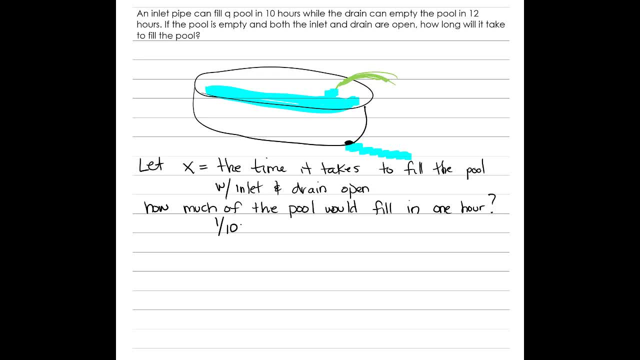 tenths filled. eighth hour: eighth tenth filled. nine hour: nine tenth filled. and in the tenth hour, out of ten tenths would be filled. in other words, ten over ten is one. it's completely filled. let's take that same idea and let's start with a field pool. 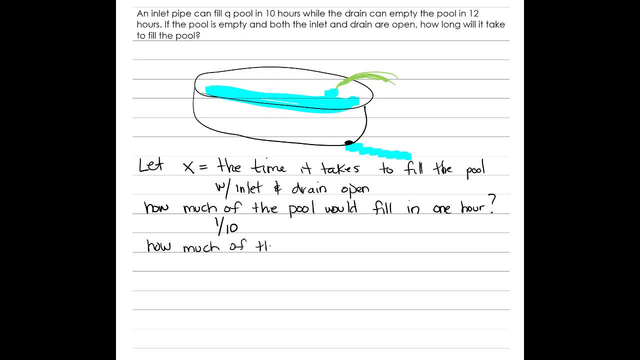 how much of the pool would drain in one hour. okay, we're starting with a filled pool and if we just let the plug out and let it completely drain, it would take twelve hours. so in one hour it would be drained 1, 12th of the way in the second hour, two twelfths, third hour, three twelfths and 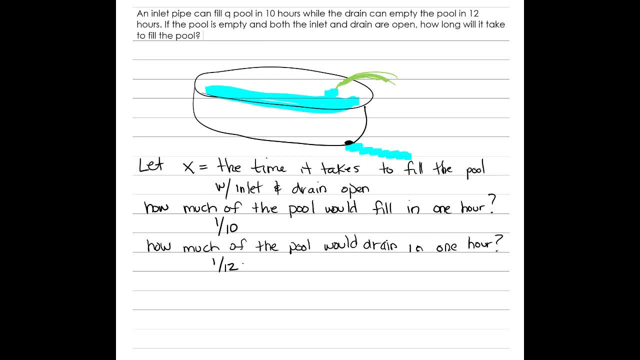 so on and so forth, until you get to the 12th hour, and now 12 12ths is drained, in other words, the whole entire pool is drained into one hour, and so on and so forth. so in one hour it would take 12, 12 hours. now, filling a pool is adding water. 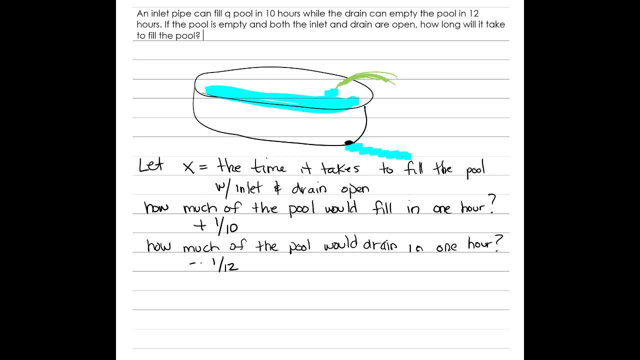 draining the pool is subtracting water. now we have both of these things going on. a pool is adding water. draining the pool is subtracting water. now, we have both of these things going on at the same time. so here's our equation: it takes one-tenth per hour to fill the 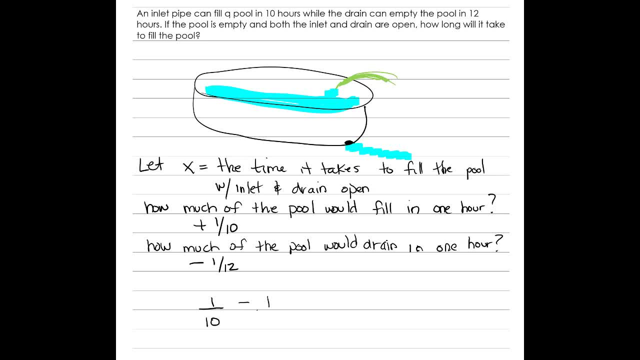 pool. we have to subtract 12 12 hours to fill the pool, and here's how we get to the 12 12 hours, The one twelfth of the pool that's leaving in the same hour. Well, how much of the pool is then filled in the one hour? 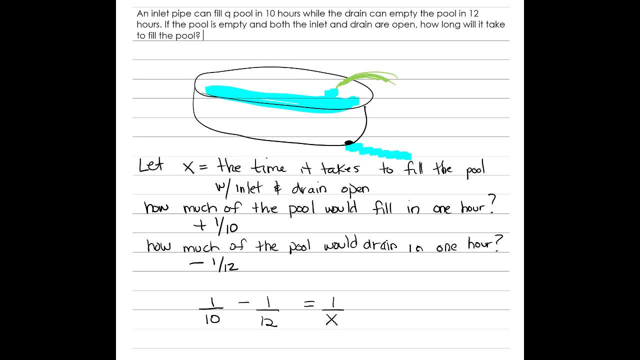 Well, that's one x of the time that it takes when both of them are going at the same time. Okay, so let me repeat this: One tenth minus, so one tenth, which is the fill rate minus the drain rate, which is one twelfth. 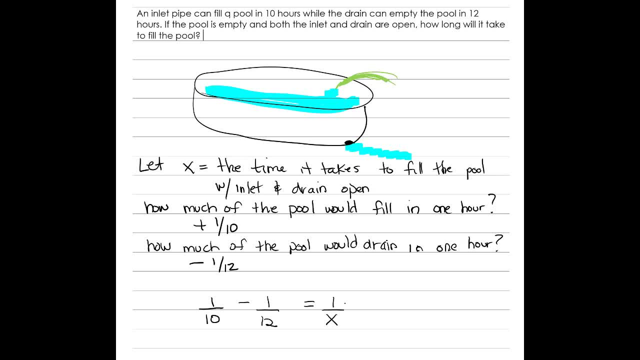 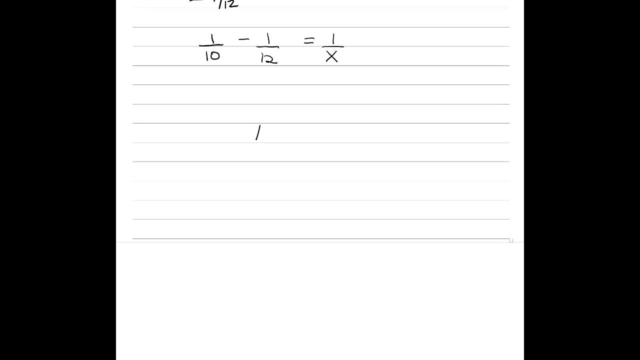 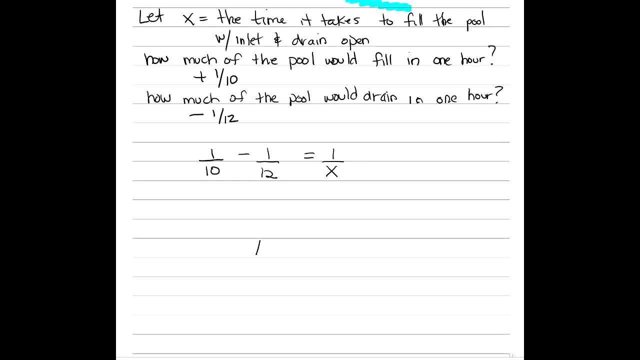 will equal when both of them are doing after an hour. Now that we have our equation, we can solve for x. Okay, let's find common sense. Well, I have a 10,, a 12, and an x, and I want to find LCD here. 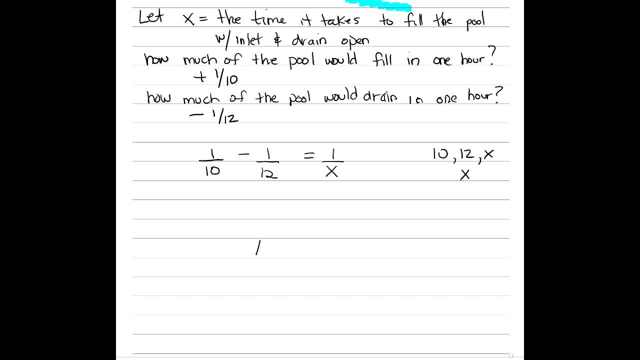 The LCD of 10,, 12, and x. well, I definitely need a 12,, I mean I definitely need the x, And the LCD between 10 and 12 is 60. So 60x is our LCD. 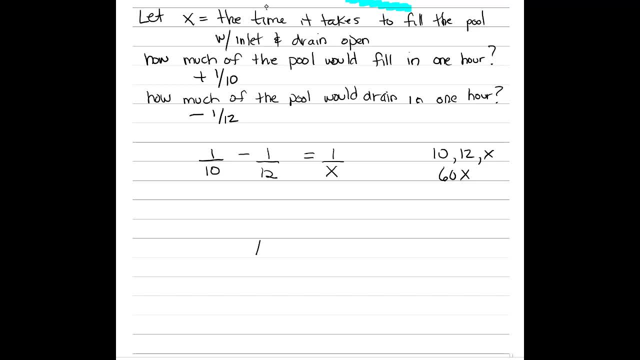 I'm going to multiply each term. I'm going to multiply each term by 60x so I can get rid of those denominators 60x, 60x and 60x. Okay, Well, 10 goes into 10 once 10 goes into 60 six times. 12 goes into 12 once 12 goes into 60 five times. 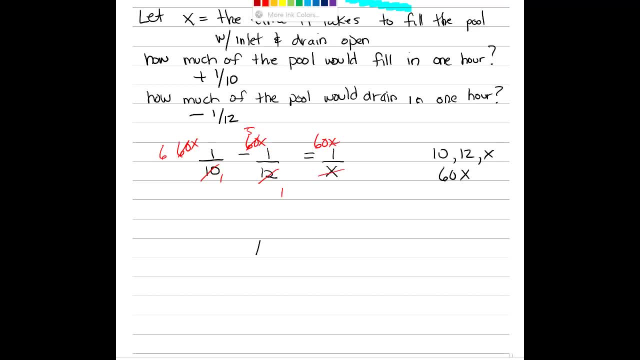 and x goes into x, once leaving 60.. So here's our new problem: 6x times 1 is 6x. minus 5x times 1 is 5x, 60 times 1 is 60.. Well, 6x minus 5x is 1x and x equals 60. 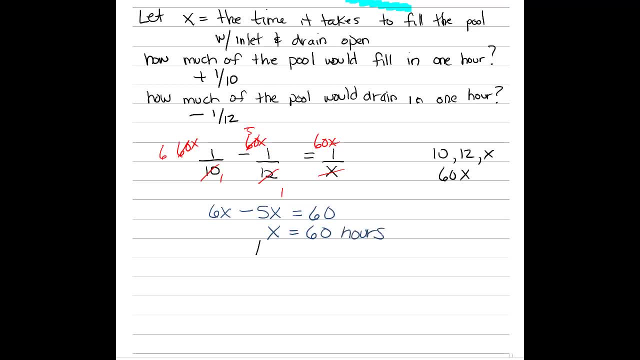 In fact 60 hours The pool will fill, but it will take 60 hours to fill If you leave both the pipe on and off at the same, or the water coming in and the drain letting it out at the same time. 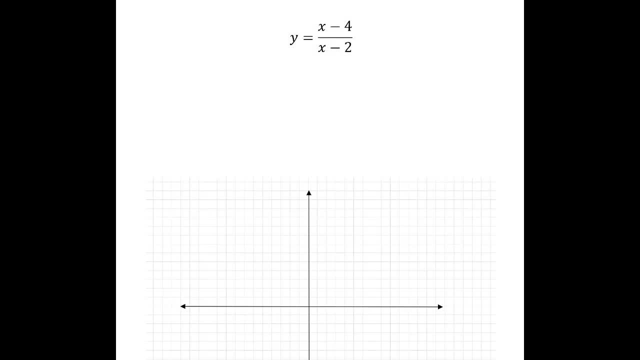 60 hours to fill. Let's take this rational function and graph our function. Okay, so there's a couple ways how we can conquer this. The first thing I want to do is I want to find the y-intercept. Okay, the y-intercept is when x equals zero. 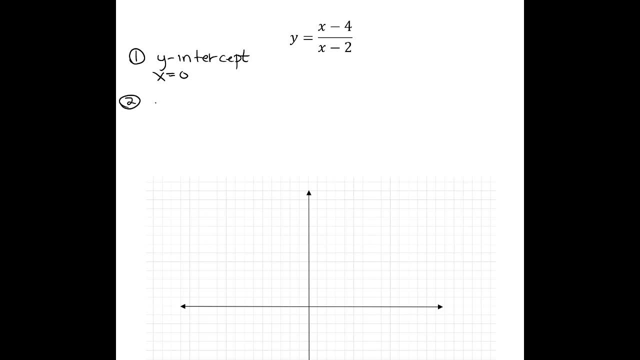 The second thing I want to graph well is the x-intercept. Well, that's when y equals zero. and then, because the x is in the denominator, We also need to figure out what is the vertical asymptote. If we have a horizontal asymptote, we'll also figure that out. 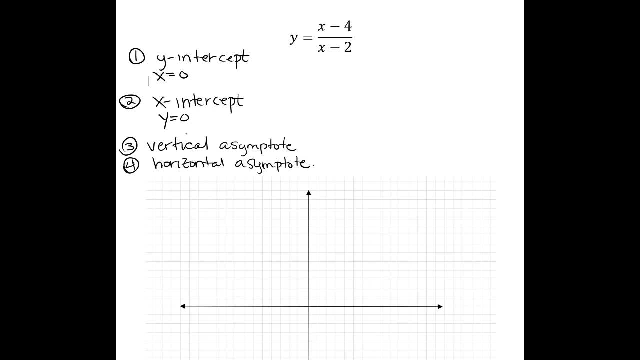 Okay, so we need to figure out these four things and then we can go from there to try and figure out what this graph looks like. Let's figure out the y-intercept. Well, that's when x equals 0, so y equals 0 minus 4 over 0 minus 2.. 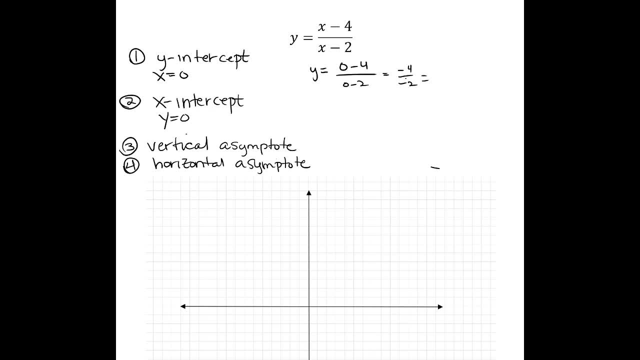 That's negative 4 over negative 2.. And well, negative cancels out the negative and that leaves us 2.. Our y-intercept is at 2.. Okay, let's check our x-intercept. Okay, well, 0, when y is 0, that's going to be x minus 4 equals x minus 2.. 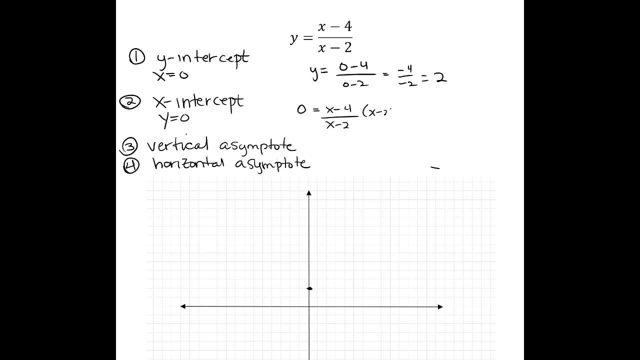 We can multiply both sides by x minus 2.. Oops, x minus 2.. Well, x minus 2 times 0 is still 0. So that gives us 0.. So that gives us 0.. So that gives us 0, equals x minus 4.. 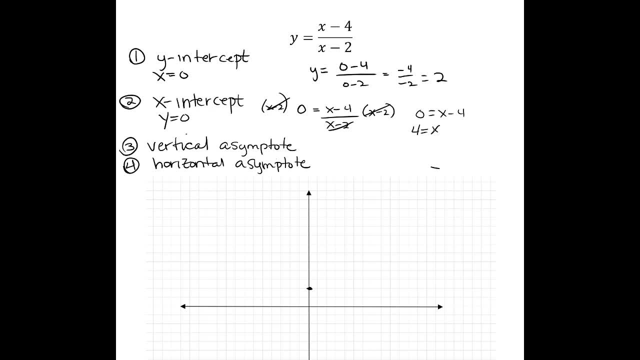 Let's add 4 to both sides. 4 equals x, So we know it crosses where x is 4.. 1, 2, 3, 4.. Okay, we know those two points. We are not connecting the dots yet. 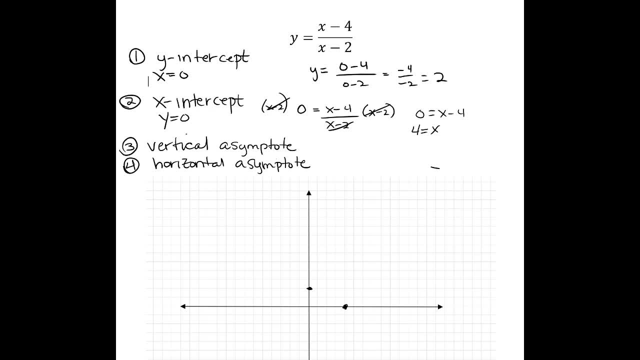 Hold on, We're not connecting the dots. What we do also need to figure out is the vertical asymptote. The vertical asymptote is when the denominator is 0.. So x minus 2, when does that equal 0?? 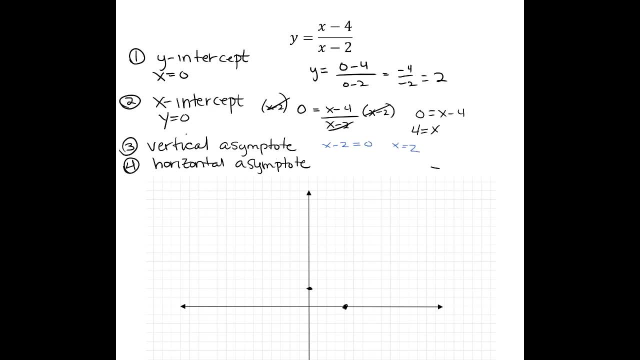 Well, when x equals 2.. Well, x equals 2 is a line. So here is our asymptote at x equals 0. Or x equals 2,, pardon me Now, horizontal or horizontal asymptote is. we're going to kind of guesstimate where it is. 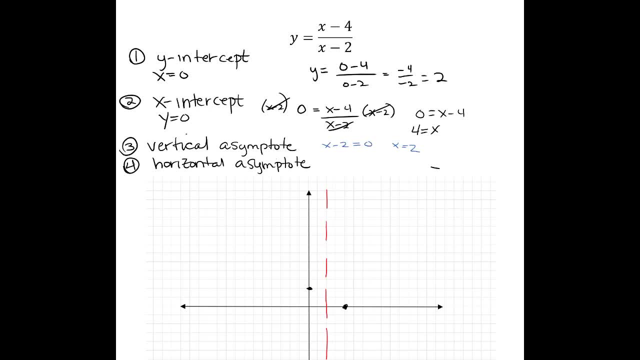 What we're going to do is choose a huge number for x And figure out what happens. Okay, so I'm just going to select 10,000 for x. Of course, it's not on my graph, But I'm going to see when I get a really, really, really big number. 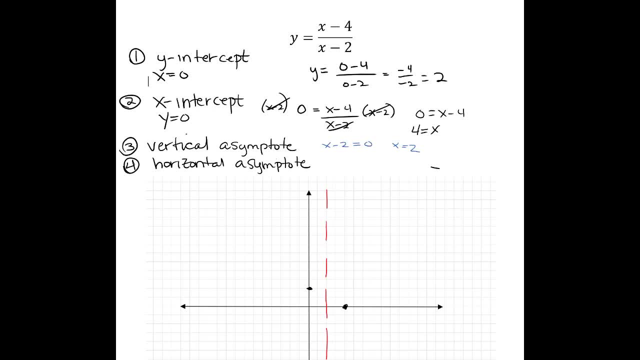 what happens to my function? Okay, y equals and I said 10,000,. you can use any big number minus 4,, all over 10,000, minus 2.. Well, 10,000 minus 4,. 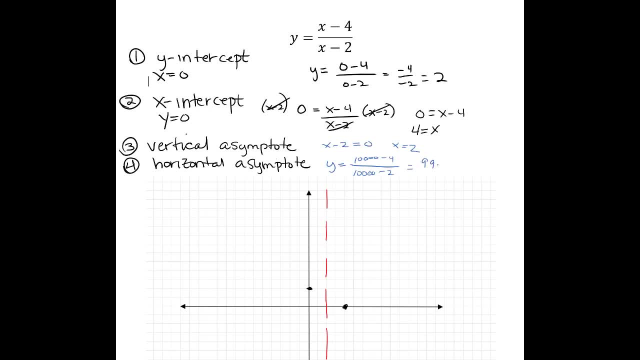 is 9,996, all over, well, 9,998.. Well, that is super-duper close to 1.. It's in fact, the larger our number gets, the closer and closer and closer it is to 1.. 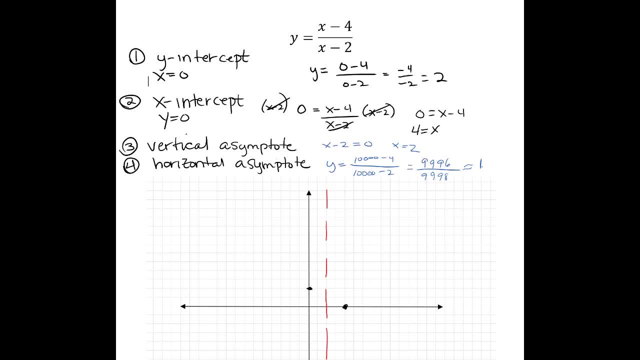 It will never be 1, but it will be very close to 1.. So the horizontal asymptote is y equals 1.. So where y equals 1 is our horizontal asymptote, We will not cross this horizontal asymptote. We will not cross this horizontal asymptote. 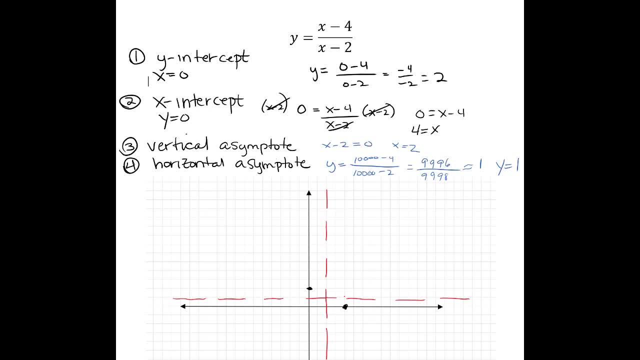 Likewise, we will not cross our vertical. Okay, now I just have to figure out some points. I'm just going to create a little table over here, my x's and my y's, and I'm going to start plugging in some values. 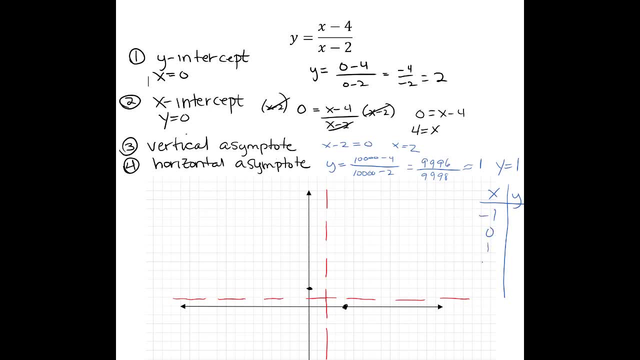 Maybe I'll do a negative 1,, a 0, a 1, a 2,, a 3,, a 4, a 5.. Okay now, when x is negative 1, you can do the math the long way. 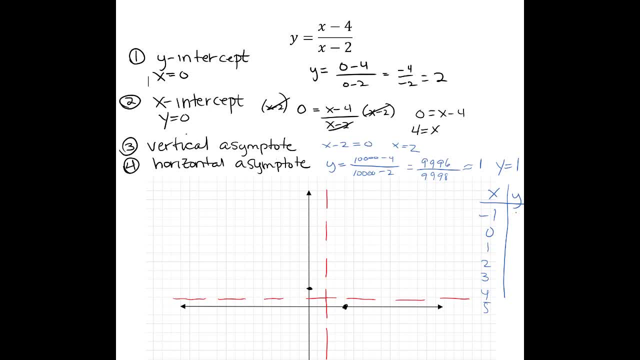 I'm just going to give you the values. When x is negative- 1,- we have 5 thirds. When x is 0, we have 2.. When x is 1,, it is a 3.. When x is 2,, the denominator becomes a 0,. 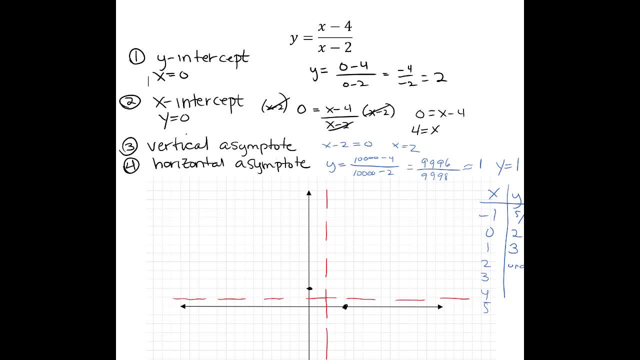 so it's undefined. When x is 3, we get a negative 1.. When x is 4, it's a 0.. When x is 5, we get a negative 1.. When x is 6, we get a negative 1.. When x is 7,, we get a negative 1.. When x is 8,, we get a negative 1.. When x is 9, we get a negative 1.. When x is 10, it's a 0.. 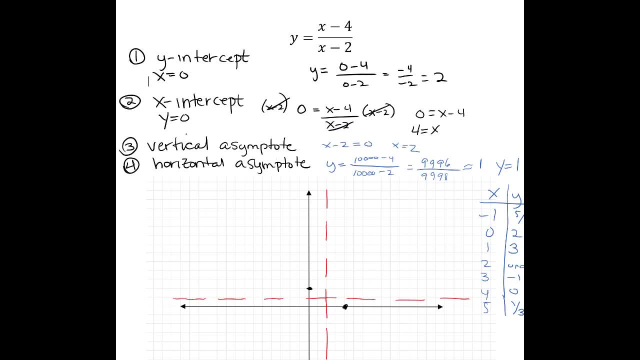 And when x is 5, it's a 1 third. These are points that we can plot Alright, so let's try it. Negative 1 and 5 thirds. Well, that's nearly 2.. It's 1 and 2 thirds. 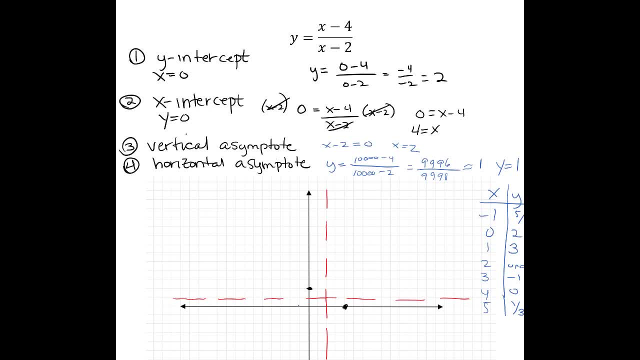 So a negative 1 and almost a 2 thirds. A 1 and 2 thirds. So that's about here. Well, that's all there is to it. Okay, now that's about it. Okay, so now that's about here. 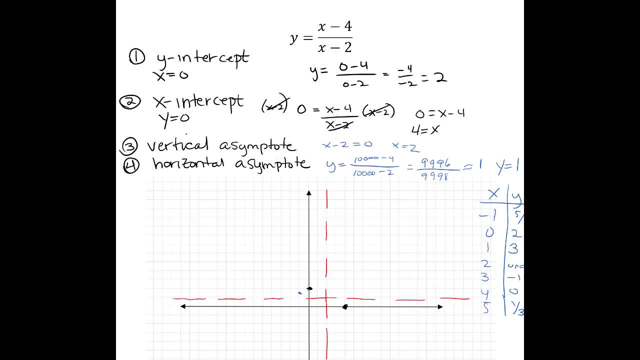 It's very close to there: A 0 and 2, we already plotted, because that's our intercept, A 1 and 3. And in fact, the closer I get the 2,, the closer it goes running off to a positive infinity. 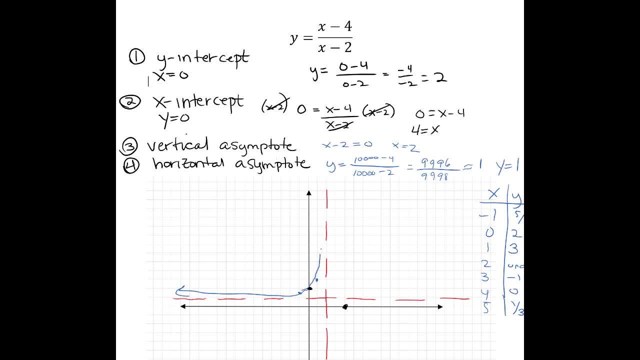 So here's our graph. You'll start to get the sense of what these graphs look like. on the left-hand side. On the right-hand side: 3 and negative 1.. 1,, 2,, 3, and negative 1.. 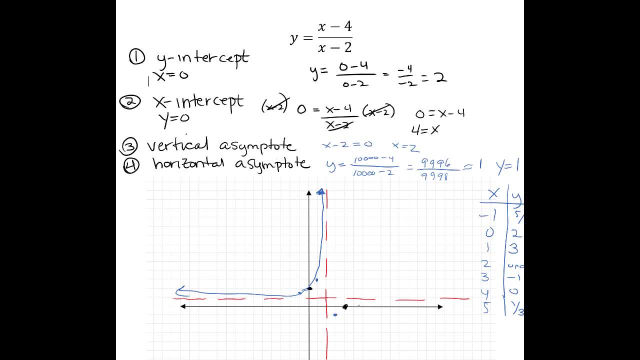 4 and 0, we already had- And 5 and 1. third is just slightly above the line. And again, it's this nice curvy shape. It never touches those red lines, but it comes very, very close. Alright, that is it for this lesson.